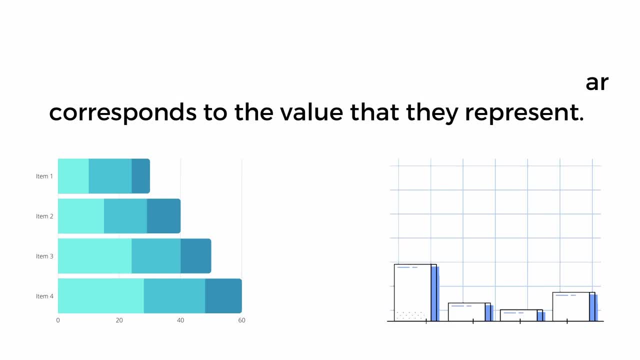 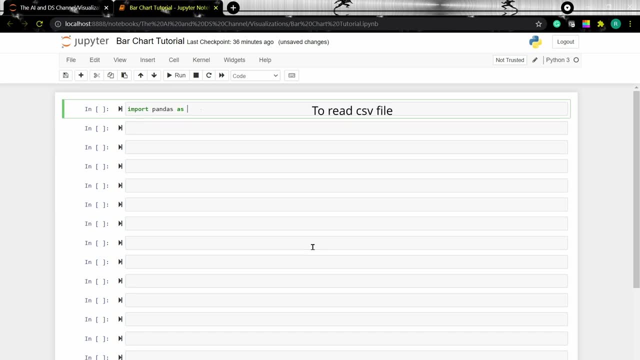 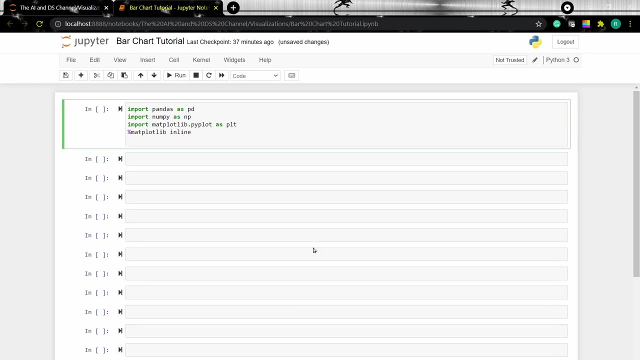 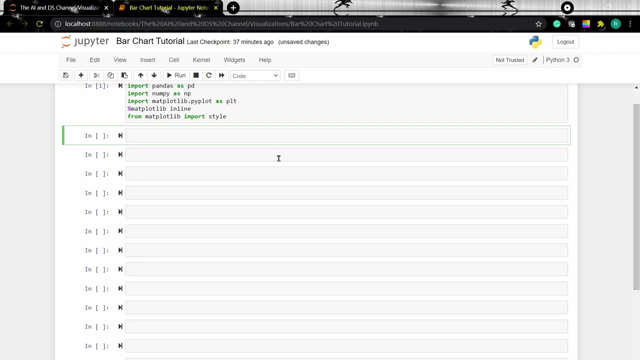 horizontally or vertically. Let's now head over to Jupyter Note. The first thing to do is to import the required libraries. So let's import the libraries Now. let's create a sample data set, The data set that we're going to create. 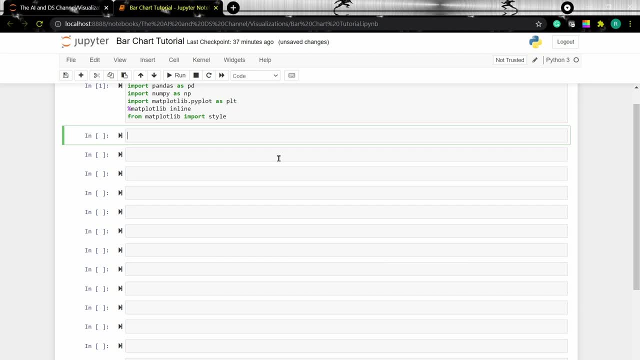 shows the average time spent by a person on different social media platforms. We'll assign this first, And the second thing to do is to name the data. The two variables we're going to use are the data set and we'll name it as the A. 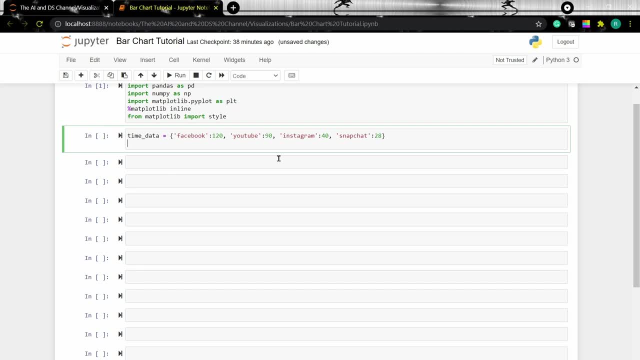 and the B, and then the A and B, and then B and B and B, and they're all the same. Now, since this is in a dictionary format, I'm going to create variables to store the keys and values separately. 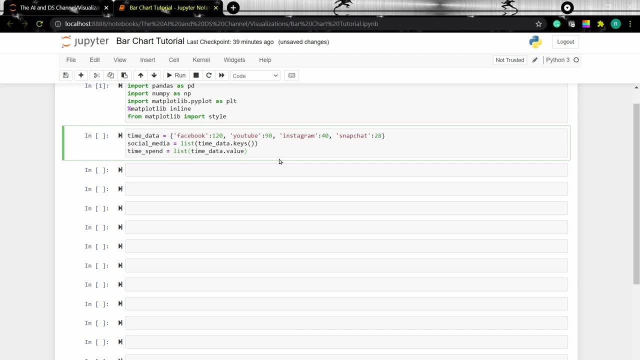 now let's create a simple bar chart. to plot a simple bar chart, we can just type in plotbar and pass our variables into it, with the second variable being the height of the bar. so which, in this case, is a time spent. now let's change the color and width of the bar. to do that, 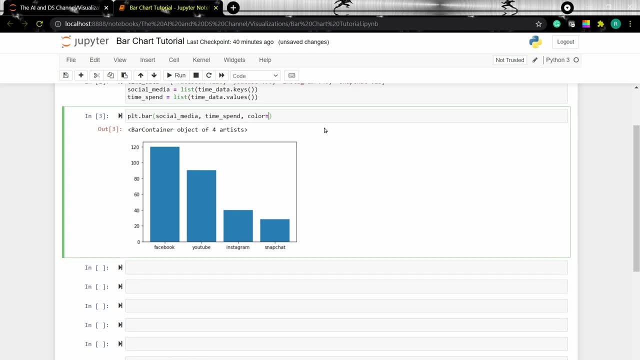 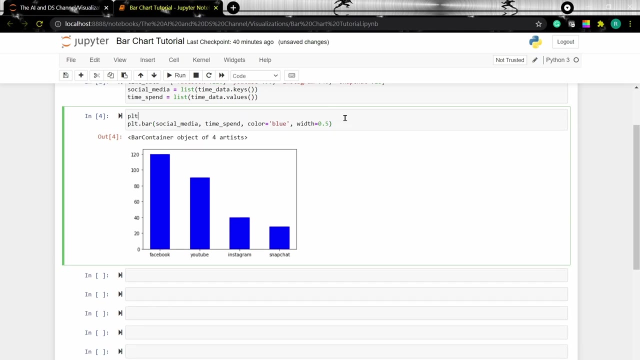 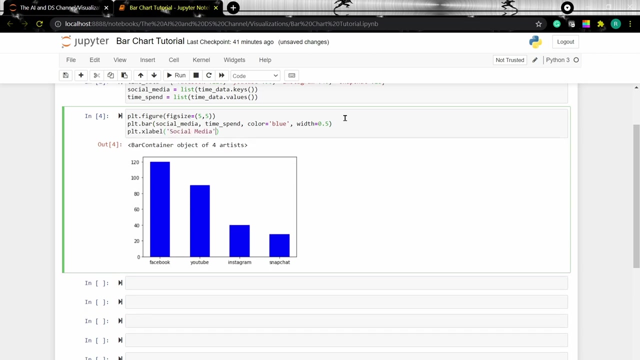 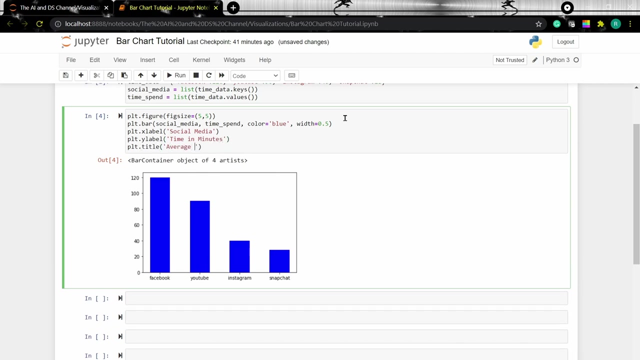 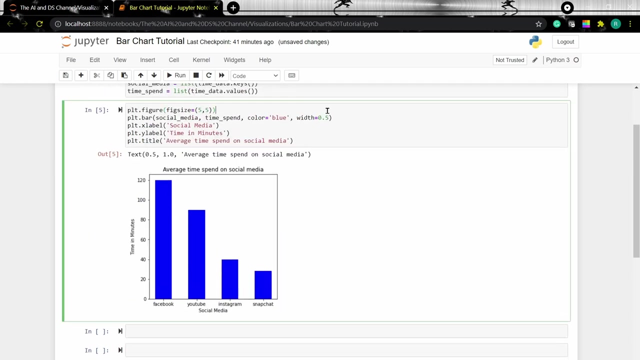 again. just type in the color and width parameters and we run the cell. we can see the color and the width has been changed. now let's change the figure size and add an x label and y label, and let's plot the graph. let's add a style to our graph. so for this i am using ggplot. 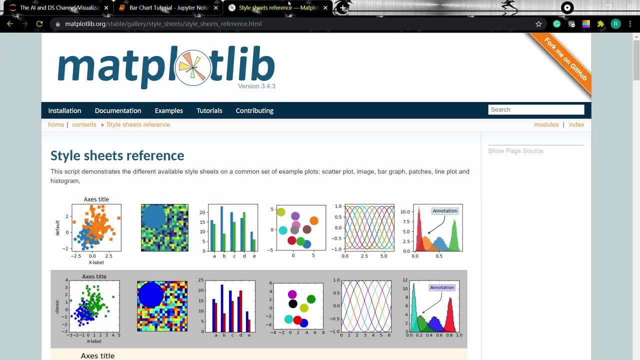 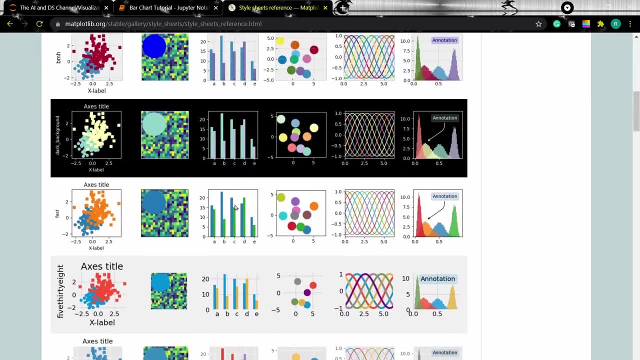 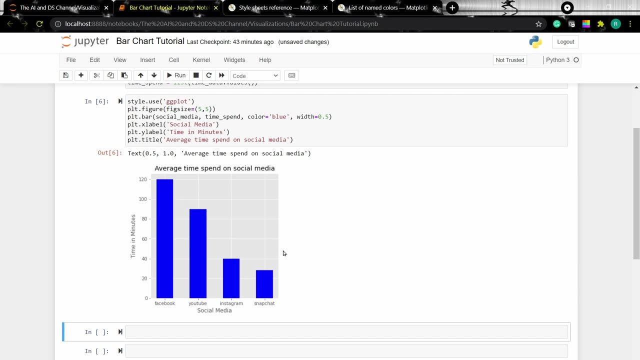 to know the different styles available for matplotlib, you can check out this matplotlib style sheet reference. i'll add a link to this in the description below. these are the different styles available for our plot. now, instead of setting a single colour, if we want to give different color of the bar, we can do that also. so for that i'm setting a variable color, which. 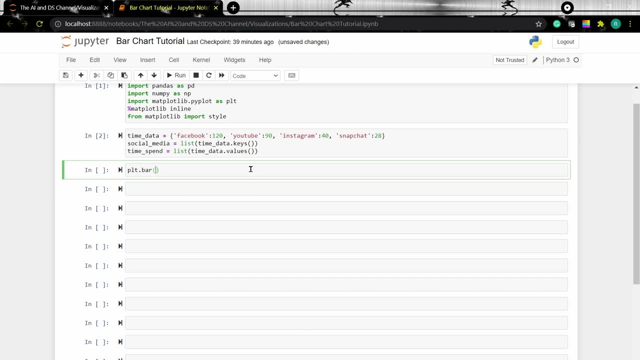 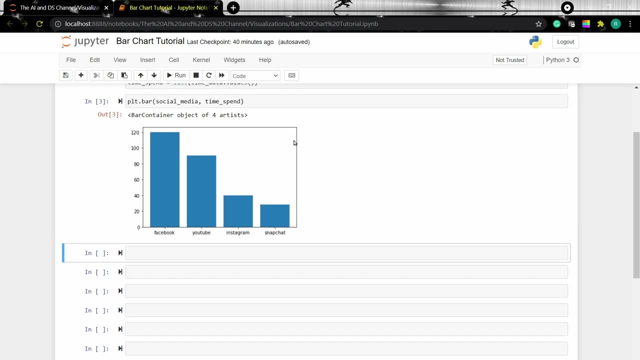 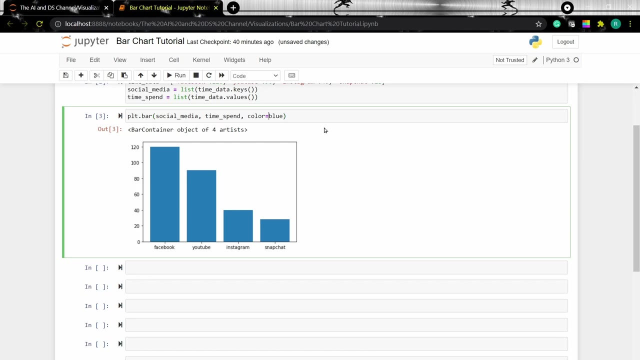 and pass our variables into it, with the second variable being the height of the bar. so which, in this case, is a time spent. now let's change the color and width of the bar. to do that again, just type in the color and width parameters and we run the cell. we can see the color and 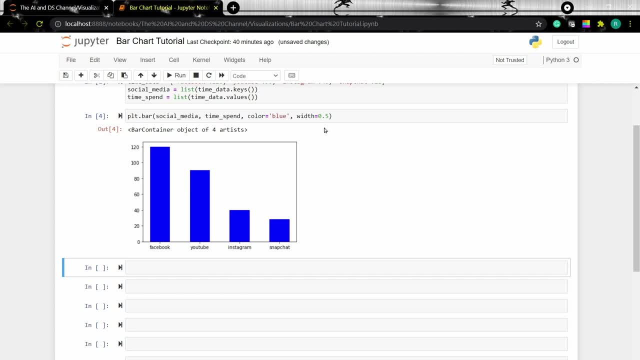 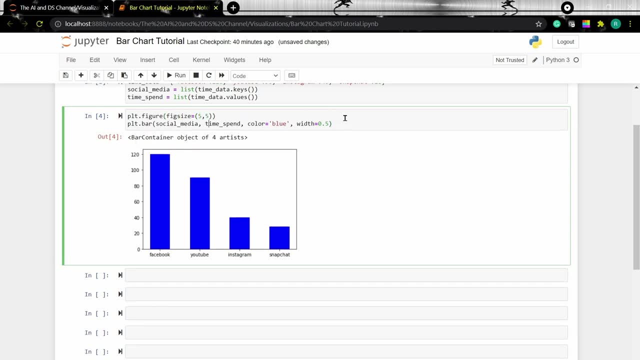 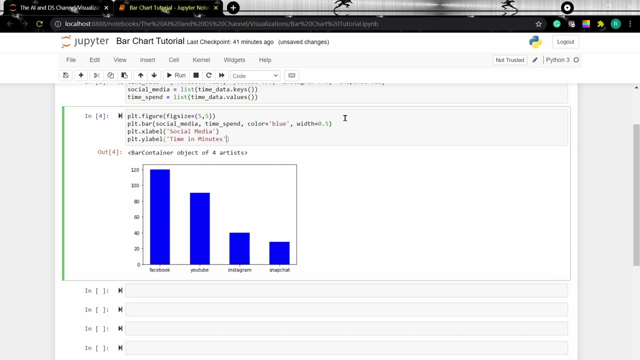 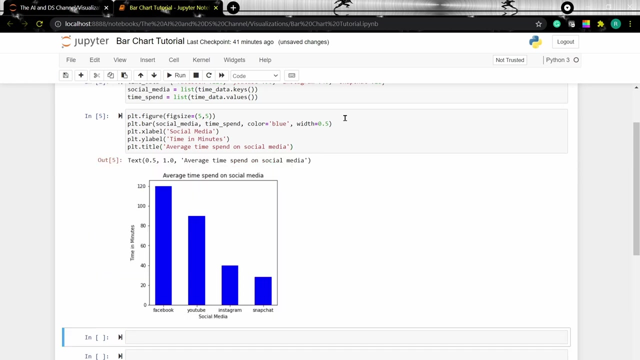 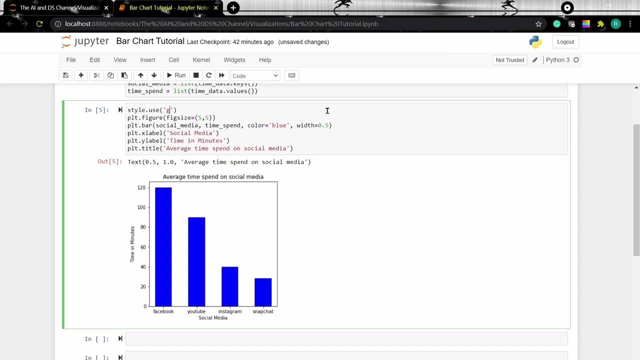 the width has been changed. now let's change the figure size and add an x label and y label, and let's plot the graph. let's add a style to our graph. so for this i am using ggplot to know the different styles available for matplotlib. you can check out this matplotlib. 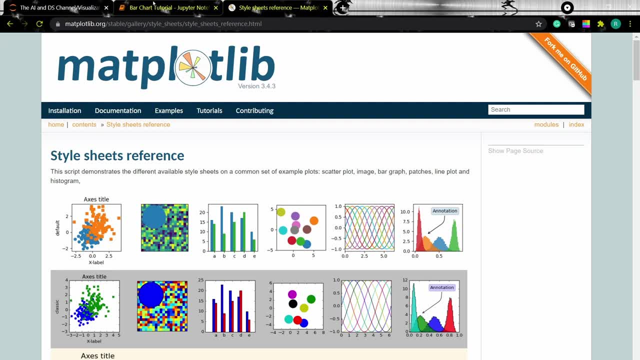 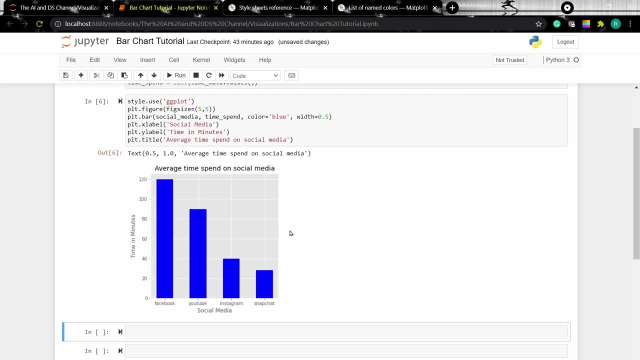 style sheet reference. i'll add a link to this in the description below. these are the different styles available for our plot. now, instead of setting a single color, if you want to give different color of the bar, we can do that also, so for that i am setting a variable color. 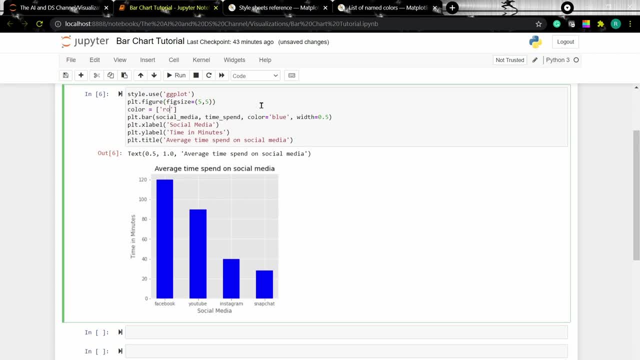 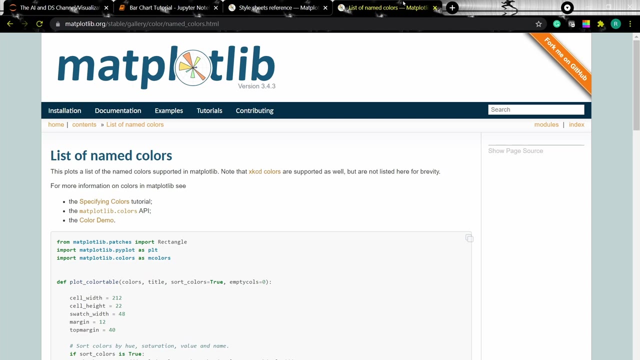 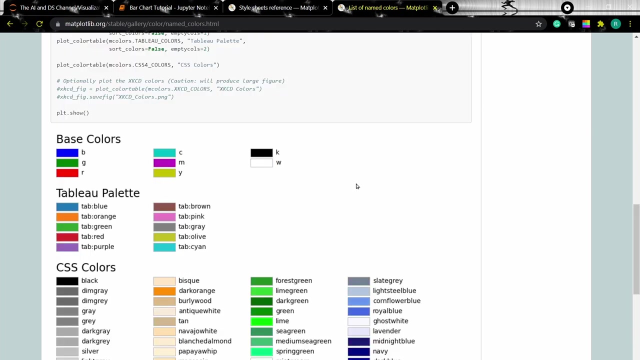 which holds a list of the different colors and i am passing the list over here. so now the different list of colors available in matplotlib. you can check out this matplotlib list of named colors and these are the different colors available for matplotlib. i'll add a link to this in the description below. 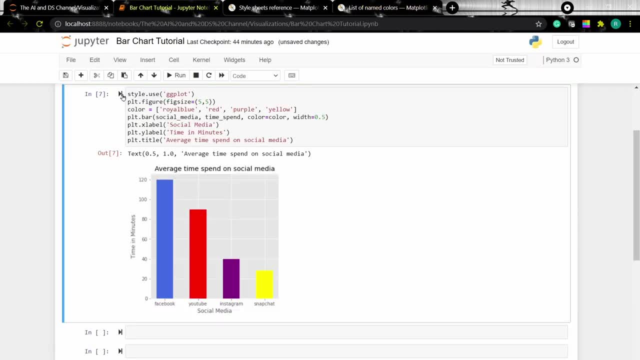 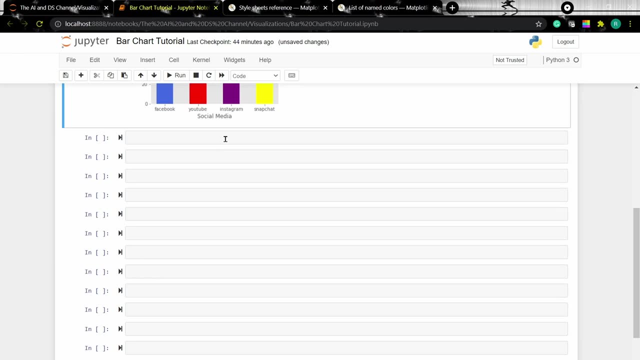 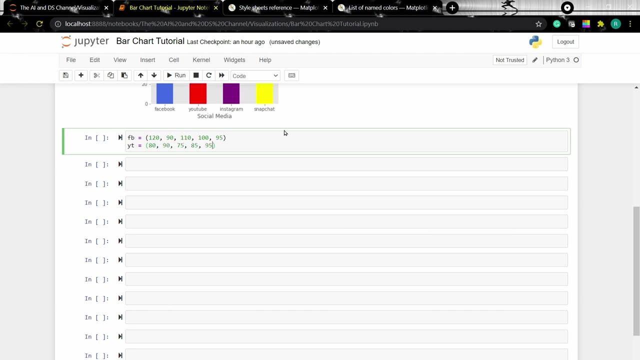 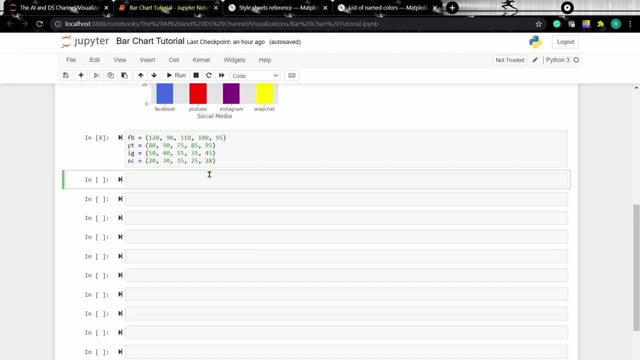 and now let's plot this and, as we can see, we have different color for our bar. now let's look at how to create a multiple bar chart. so first we'll create a data for a multiple bar chart. so this is our data for our bar chart. now we need to arrange the data on the x-axis. 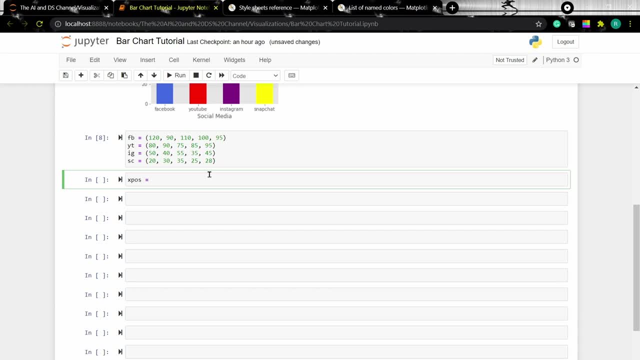 so to do that, let's define our x-axis. we need some data for our bar chart, so we need to, in the x position, numpy dot, arrange length of our data. so what this will do is it'll arrange the data on the x axis and to see x pos, we can just type in x pos. 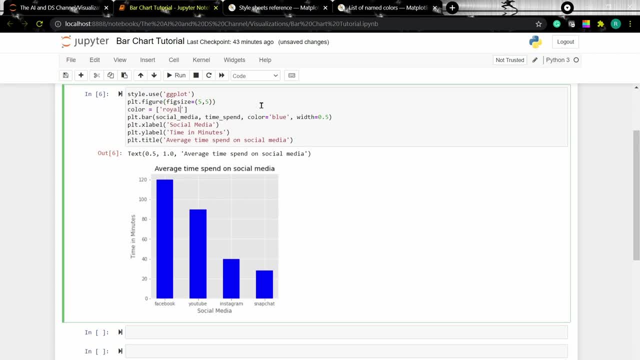 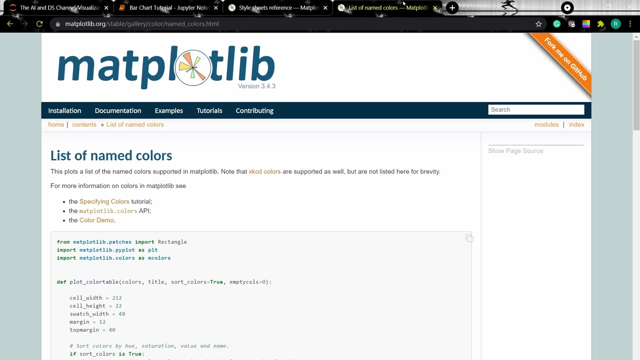 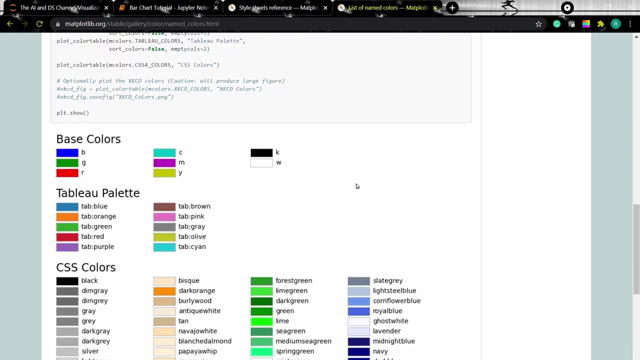 holds a list of the different colors and i'm passing the list over here. to know the different list of colors available in matplotlib, you can check out this matplotlib list of name colors and these are the different colors available for matplotlib. i'll add a link to this in the description below. and now let's plot this and, as we can see, we have different. 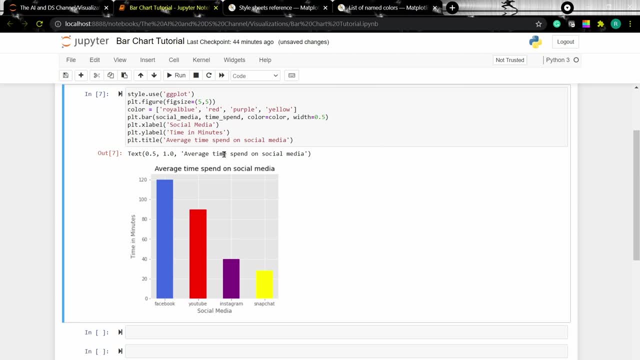 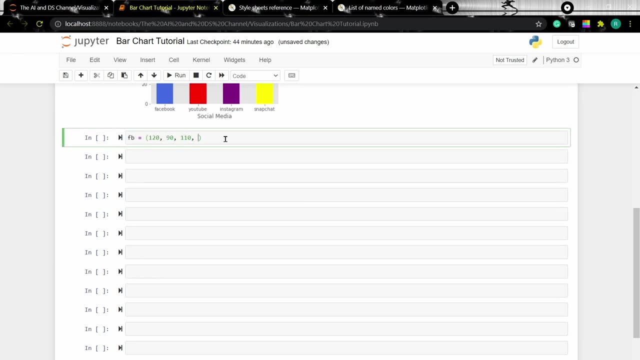 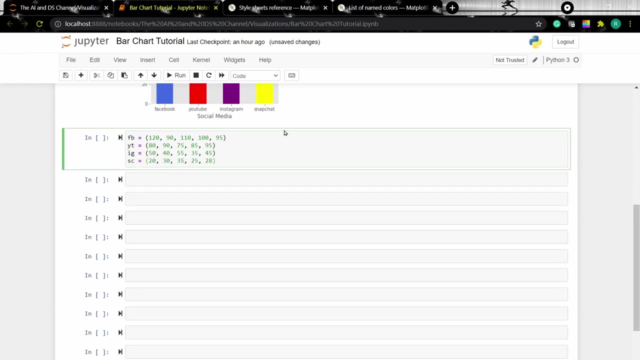 color for our bar. now let's look at how to create a multiple bar chart. so first we'll create a data for a multiple bar chart. so this is our data for our bar chart. now we need to arrange the data on the x-axis. so to arrange the data, we're going to click color x in eraser first and then taste to see if it works. 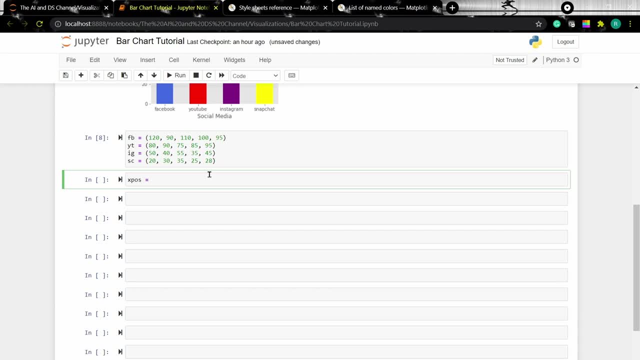 our chart. so this is change for our data screen. click on add to scene. so the best way to do it is to give you an example of the block number and check these, because same font name and this is ok, like a. do that. let's define the x position. numpy dot- arrange length of our data. so what this will do. 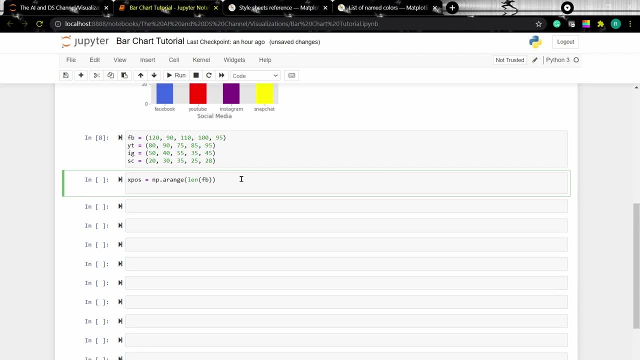 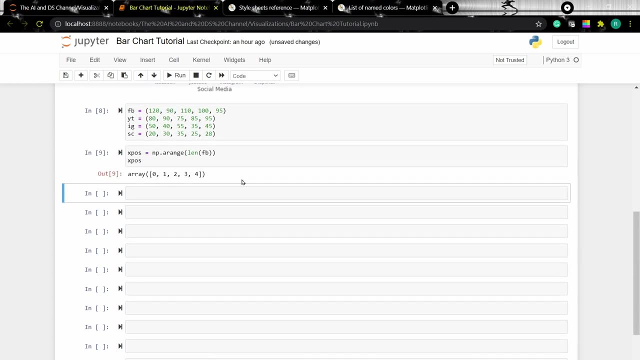 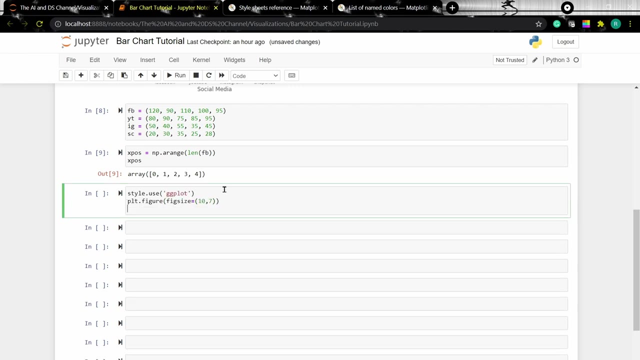 is. it'll arrange the data on the x axis and to see x pos, we can just type in x pos and you can see the array. now let's set the style, figure size and bar width for our plot. now let's pass in the data for plotting the bar. 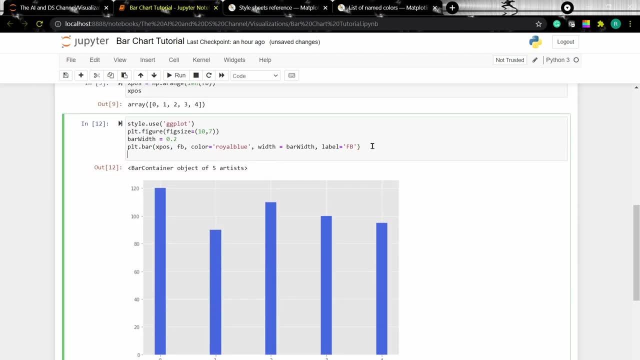 so this is our first data. now let's plot the second data. what we need to modify is we need to add a small value over here. so we need to add a small value over here. This is because, if we plot the graph, we can see that both the data will be overlapped. 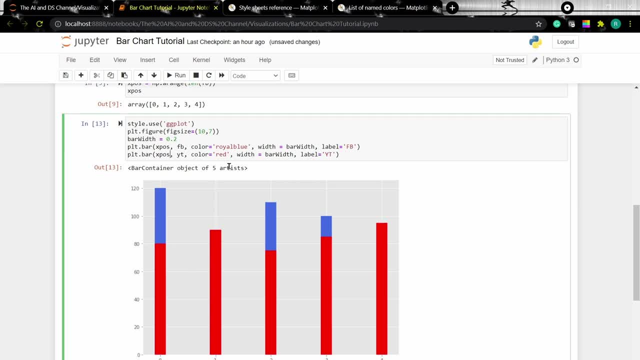 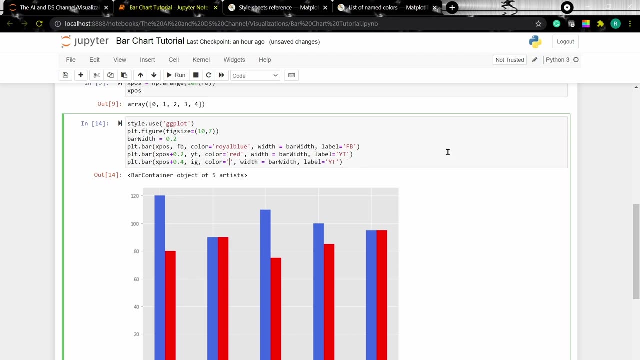 To change the position, we need to add a small value over here. Let's say 0.2.. So, as you can see, now the bars are shifted. So, similarly, let's plot the other two data. Now what this will do is the first bar will be in X position and the second bar will be at 0.2 from X position. 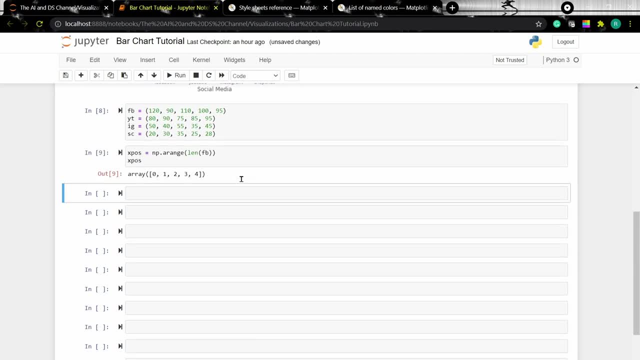 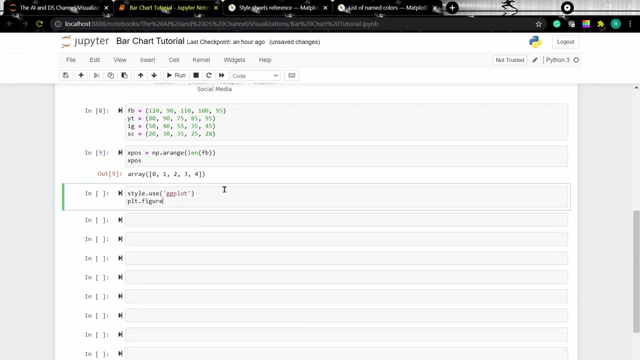 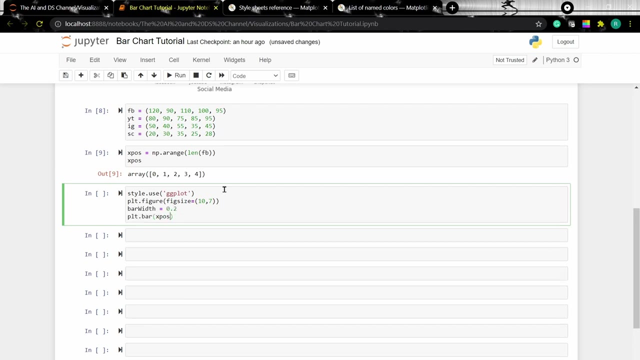 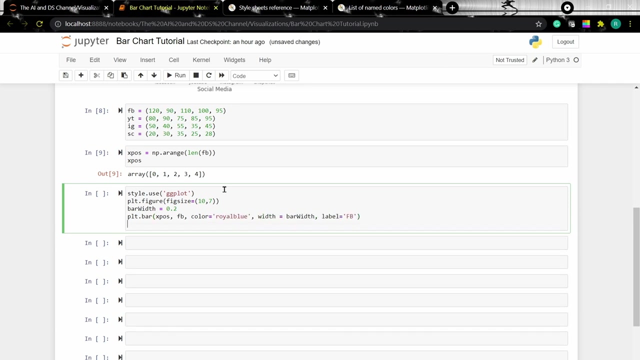 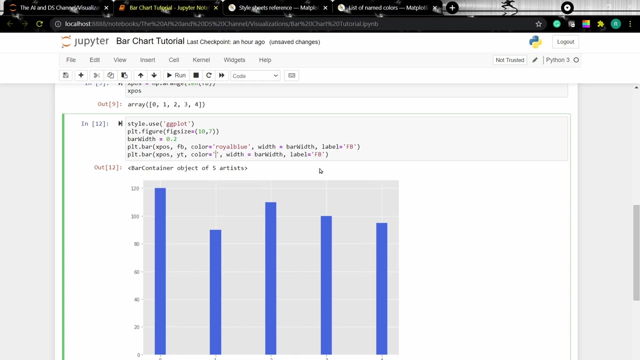 and you can see the array. now let's set the style, figure size and bar width for our plot. now let's pass in the data for plotting the bar. so this is our first data. now let's plot the second data. what we need to modify is we need to add a small value over here. 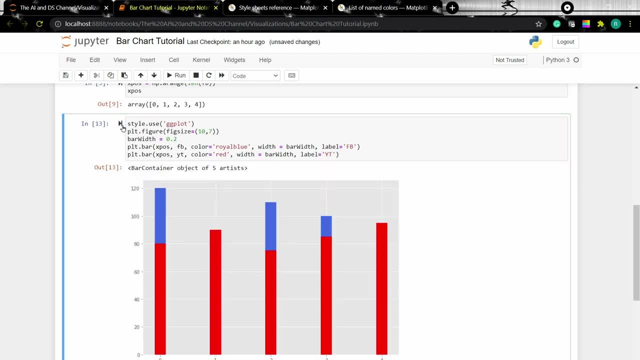 so we need to add a value over here. so we need to add a value over here. this is because if we plot the graph, we can see that what the data will be overlapped. to change the position, we need to add a small value over here, let's say 0.2. 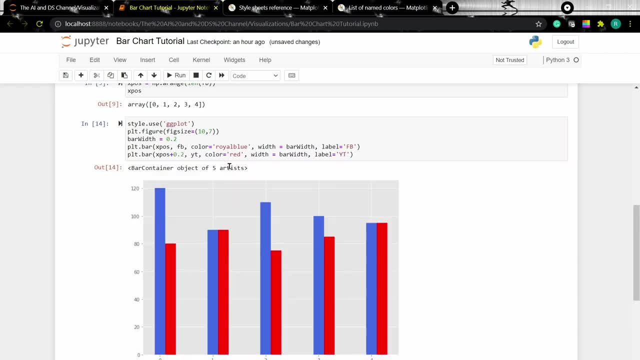 so, as you can see, now, the bars are shifted. so, similarly, let's plot the other two data now. what this will do is the first bar will be in x position and the second bar will be at 0.2 from x position, the third bar will be 0.4 from x position and the fourth bar will be 0.6 from x position. 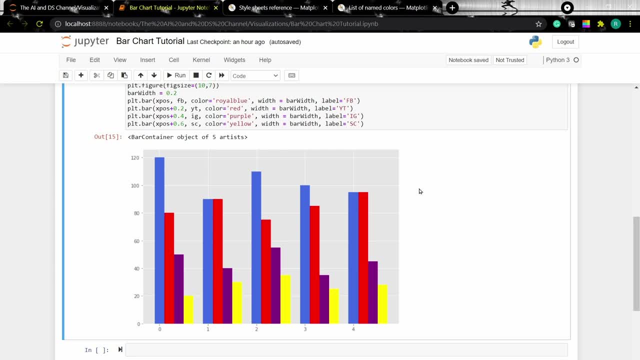 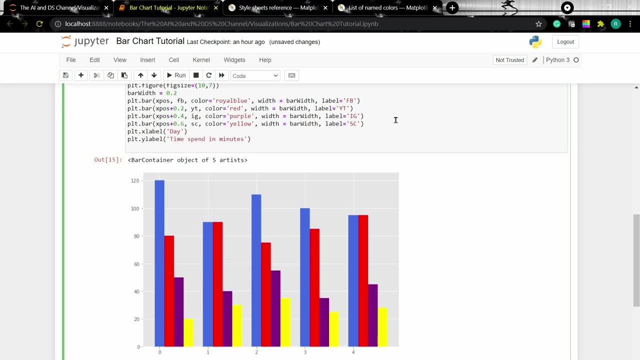 and when we run it we can see that now let's add the x label, y label and the title to plot the legend. we can type in plot dot legend and we can see that the data is now overlapped to the x label and the y label. 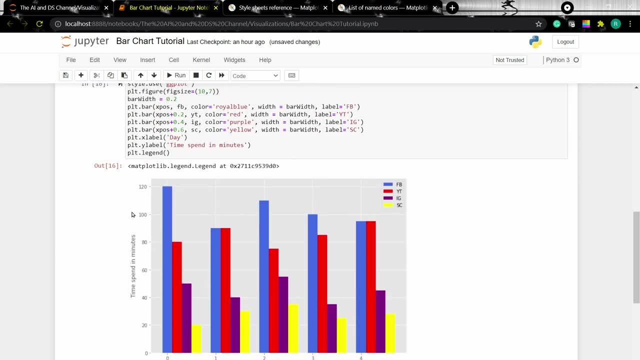 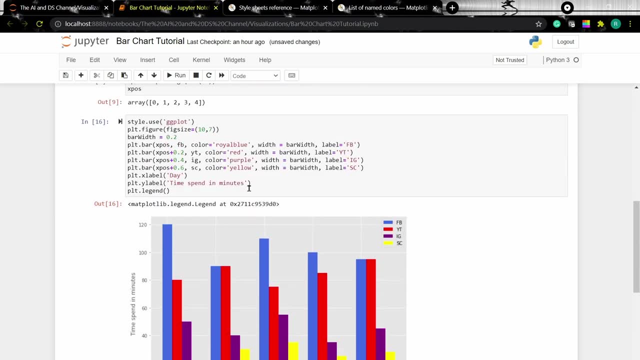 and if you run the cell we can see the titles with the legends. now we need to add in the days over here, so to do that we can type in x sticks and the position where we want to set the labels. so i'm adding a value to expose. 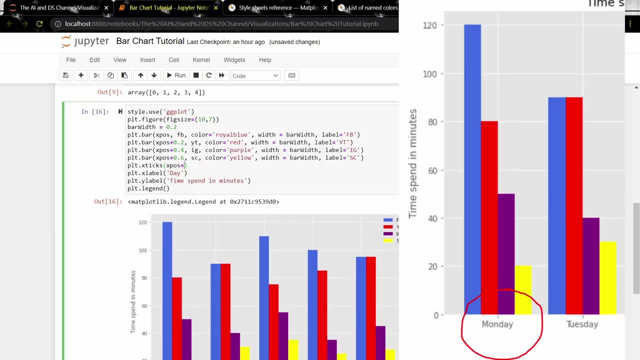 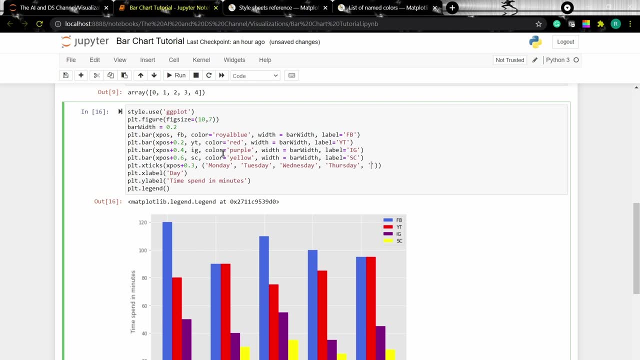 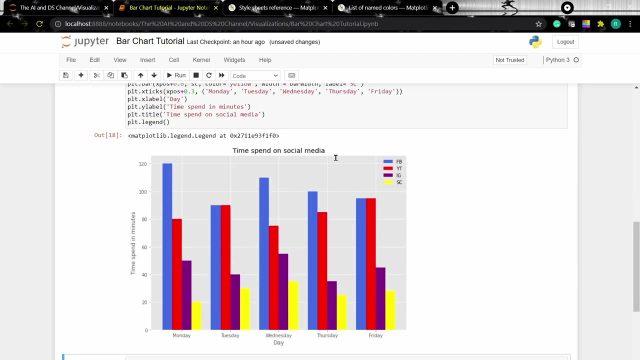 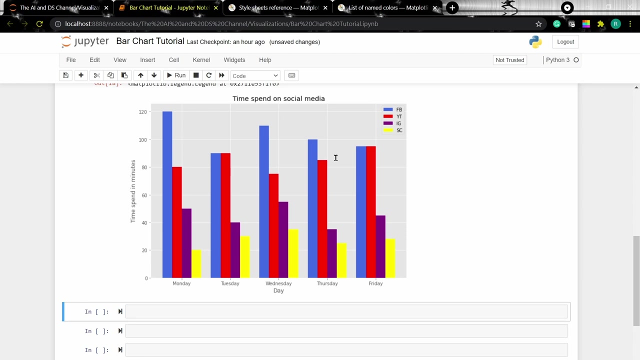 because expose is at the center and if i add a value to it, i can push it here. let's add a title and there we have a graph. now let's look at how to create a stacked bar chart. for stacked bar chart, i'm using data of two social media apps. 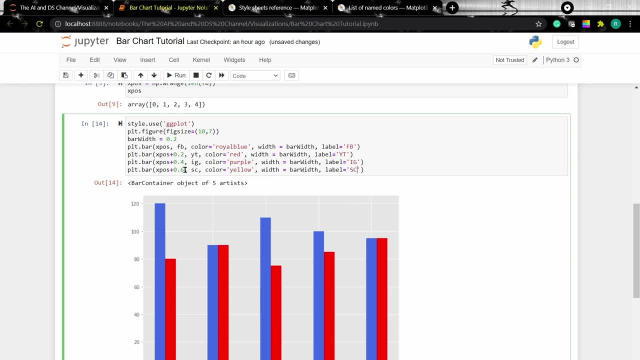 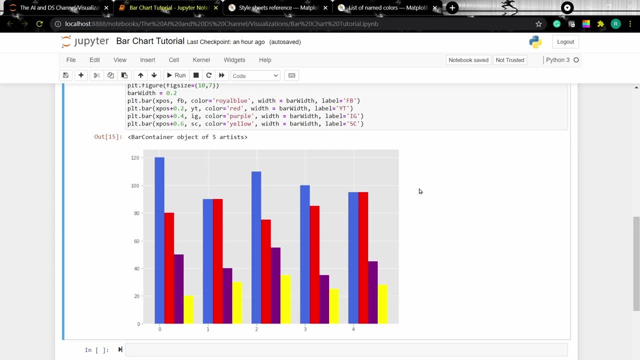 The third bar will be 0.4 from X position and the fourth bar will be 0.6 from X position And when you run it we can see that. Now let's add the X label, Y label and the title. 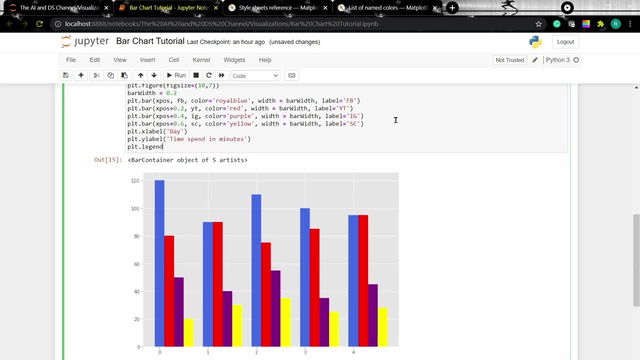 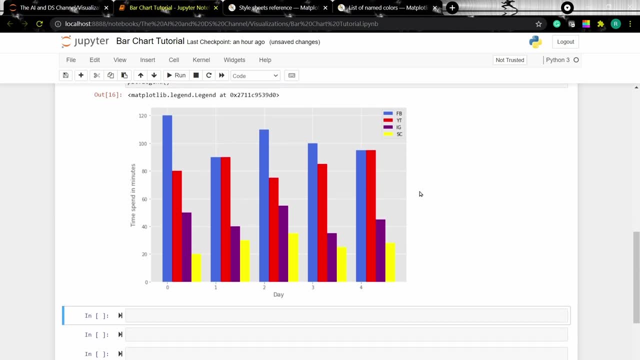 To plot the legend we can type in plotlegend And if you run the cell we can see the titles with the legend. Now we need to add in the days over here. So to do that we can type in X ticks. 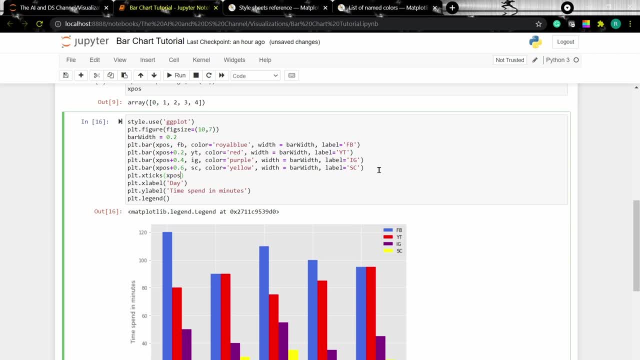 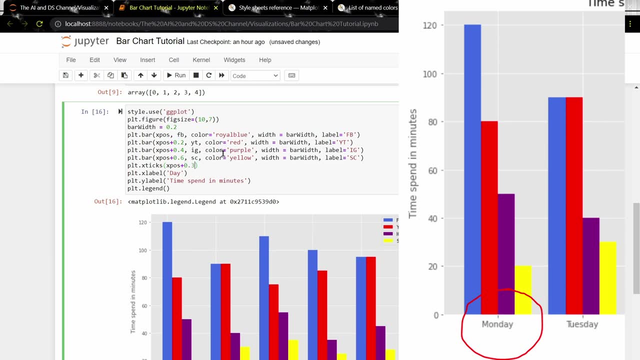 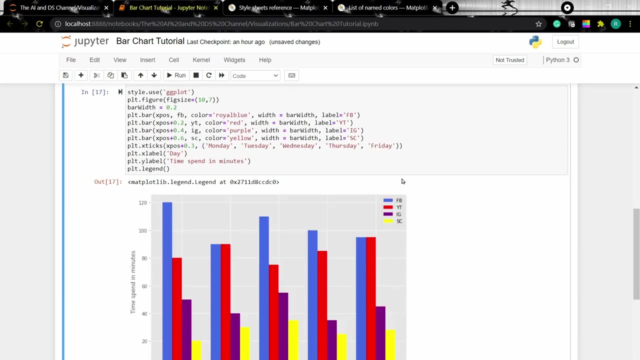 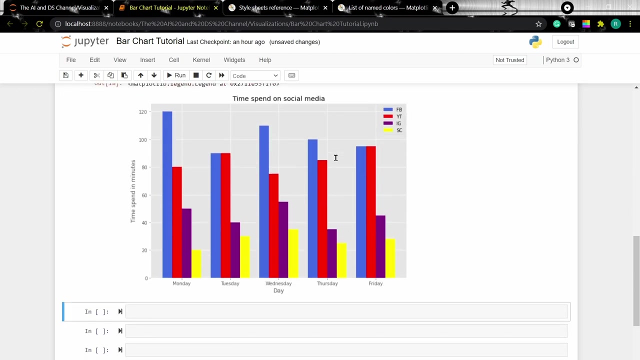 And the position where we want to set the labels. So I'm adding a value to X pose, because X pose is at the center And if I add a value to it I can push it here. Let's add a title and there we have a graph. 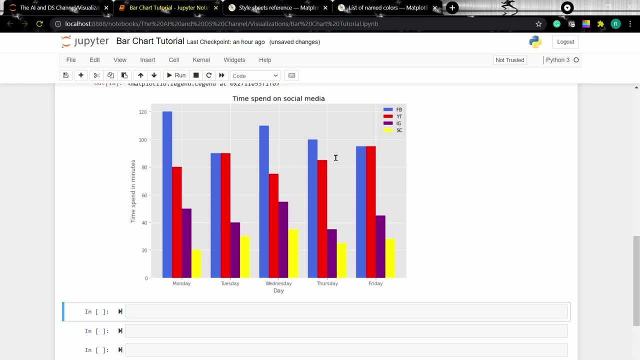 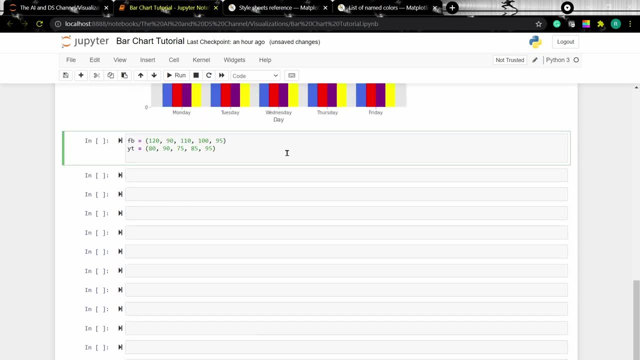 Now let's look at how to create a stacked bar chart. For a stacked bar chart, I'm using data of two social media apps. Now here I'm passing the days as a list. Now, similarly, let's arrange the data using X. 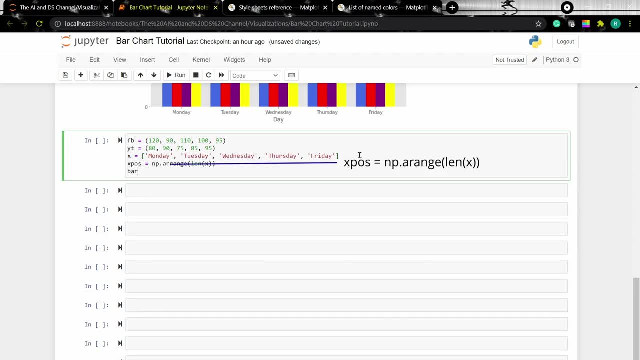 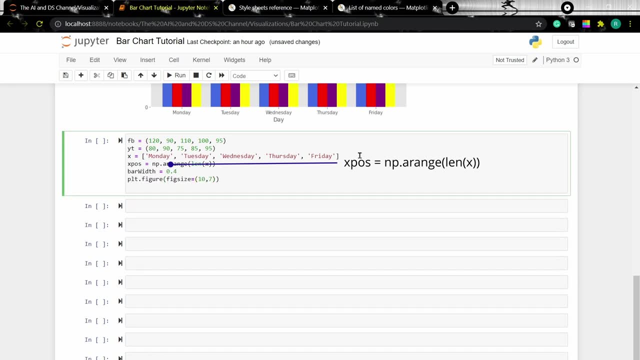 So I'm going to use X position. Now I'm going to use X position. So I'm going to use X position. Let's add the bar width Now. let's pass the data to plot the graph. Now let's add the second data. 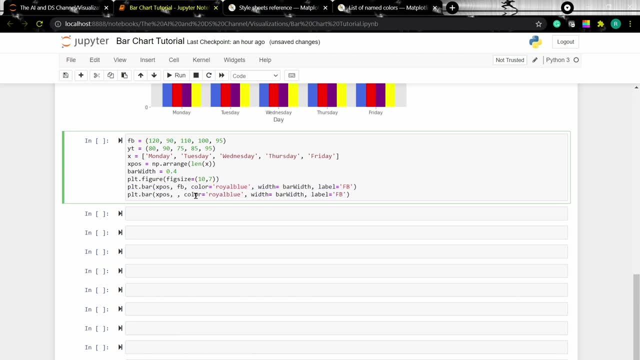 Now, let's add the second data. Now, let's add the second data. Now, since this is a stack. Now, since this is a stack bar chart, we do not need to add a value to change the position on the X axis, but we need to set the bottom variable for the second data. 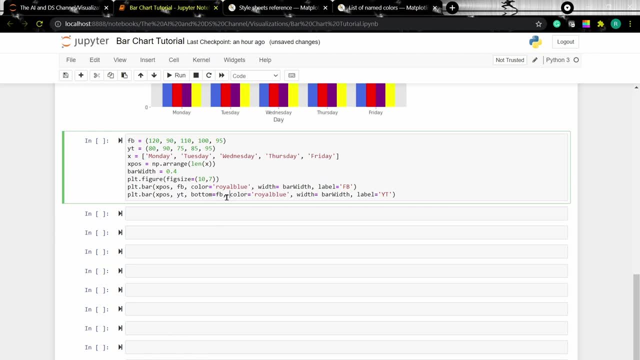 So what this variable will do is it will tell the second data to start after the first data, which in this case is FB. So if you want to plot three bars, the bottom of the third bar should begin at the second bar. 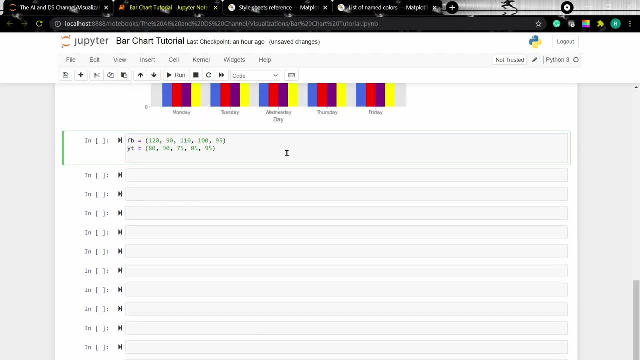 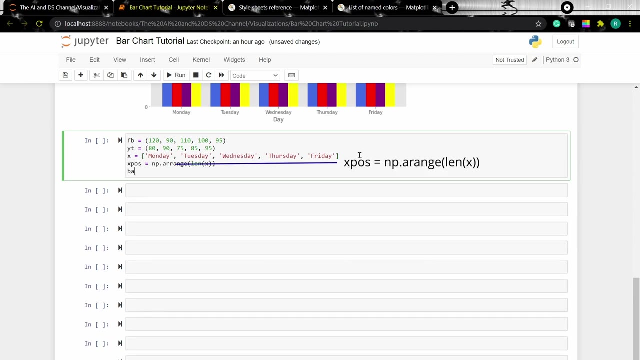 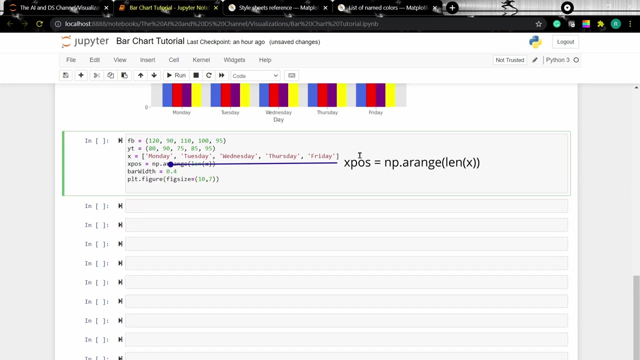 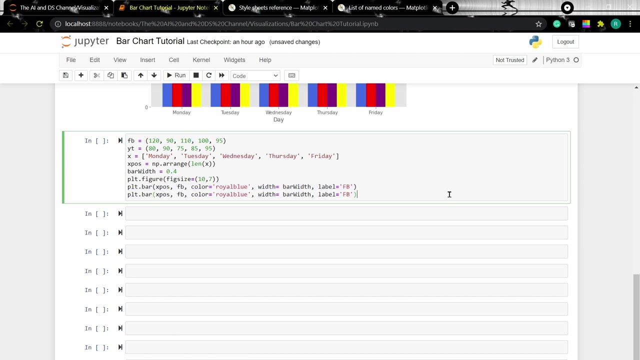 now. here i'm passing the days as a list now. similarly, let's arrange the data using expose exposition. let's set the bar width now. let's pass the data to plot the graph. now. let's add the second data now. since this is a stacked bar chart, we do not need to add a value to change the position on the x. 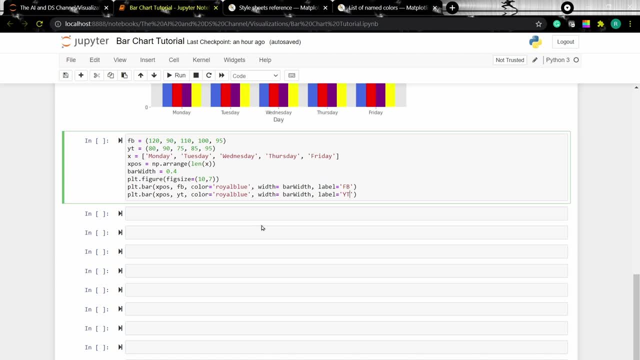 axis, but we need to set the bottom variable for the second data. so what this variable will do is it will tell the second data to start after the first data, which in this case is fb. so if you want to plot three bars, the bottom of the third bar chart will be the first bar. 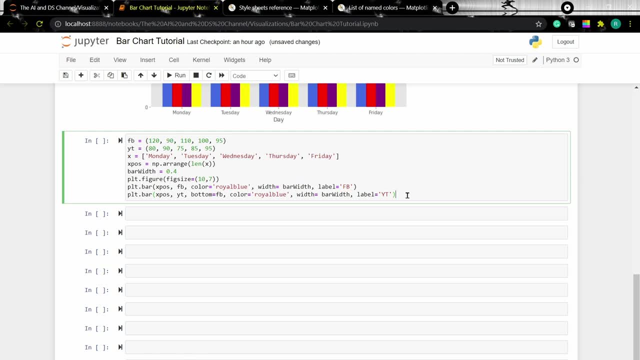 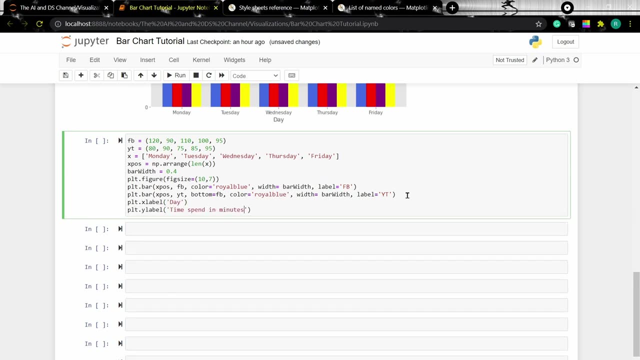 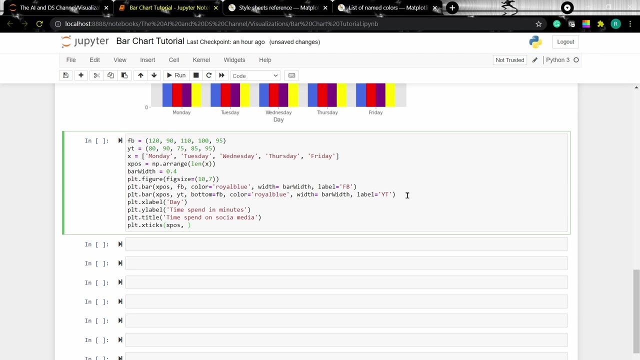 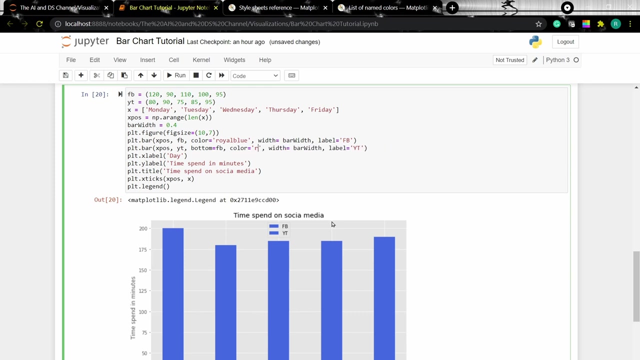 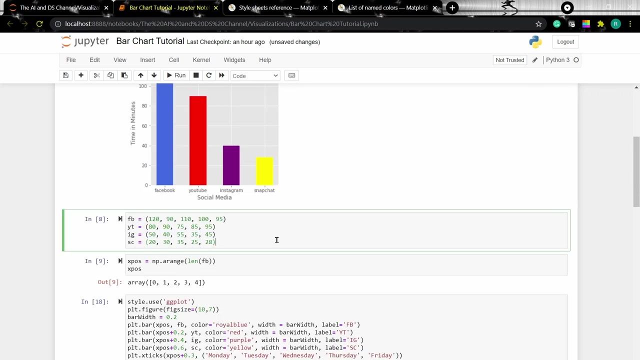 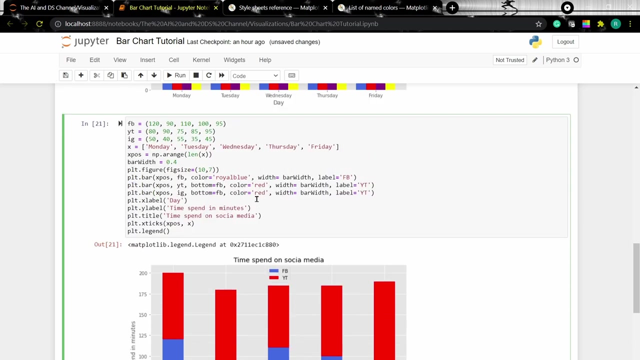 should begin at second bar. Now let's plot the title xlabel and ylabel, xpos, and here we can pass the array plotlegend to show the legends. So now we have a stat bar charts. Now let's add a third bar to this. So I am modifying the data over here. So the bottom. 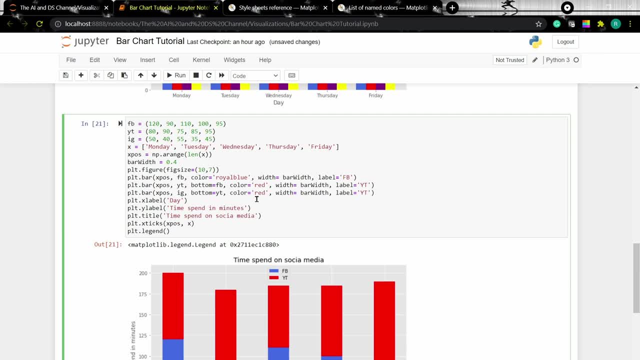 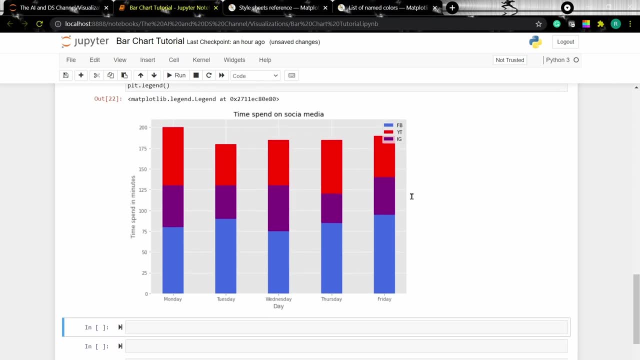 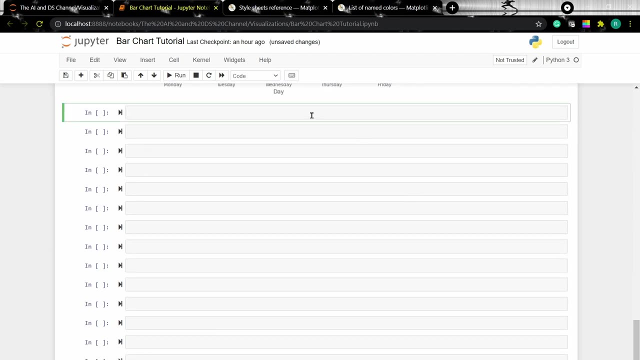 of the third bar will be the top of the second bar. that is yt. Change the color. and if you run this l, we have a stat bar chart. Now let's look at plotting data from a csv file. Now, since we have already imported pandas, I am just changing the part directory, So I am 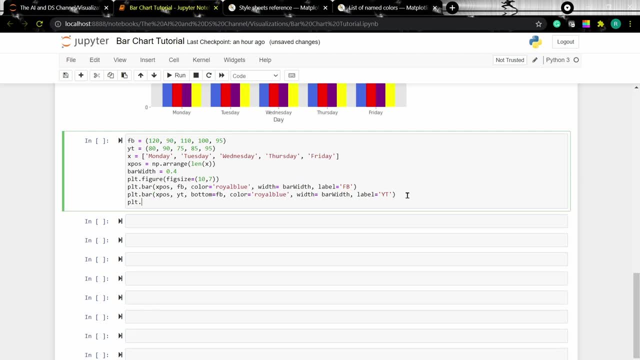 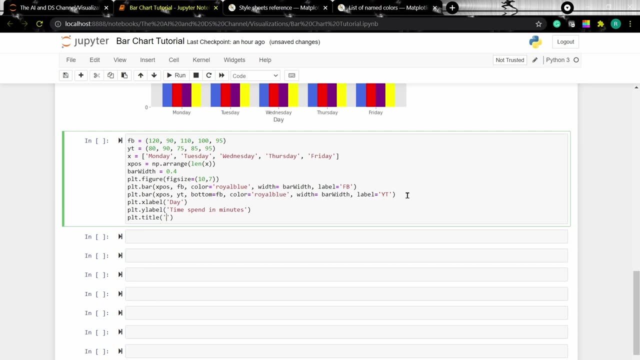 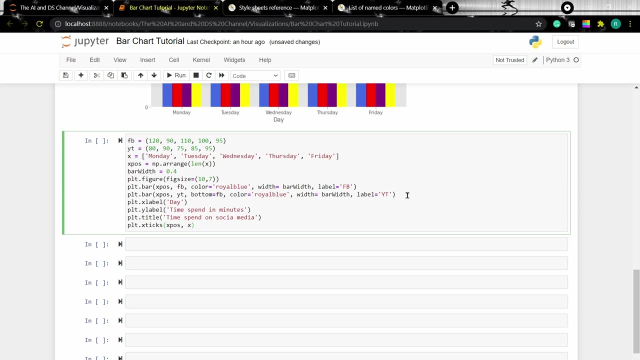 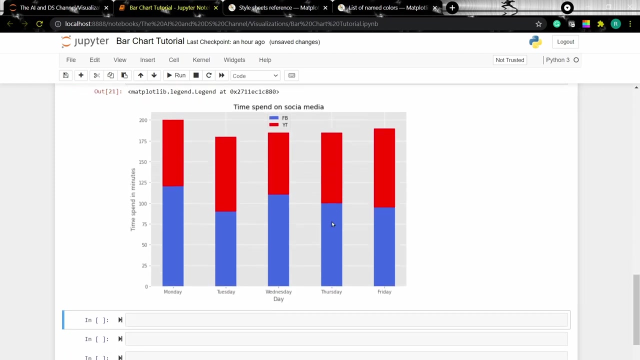 Now let's plot the title X label and Y label. Now let's plot the title X label and Y label, X, pos, and here we can pass the array Plotlegend to show the legends. So now we have a stack bar charts. 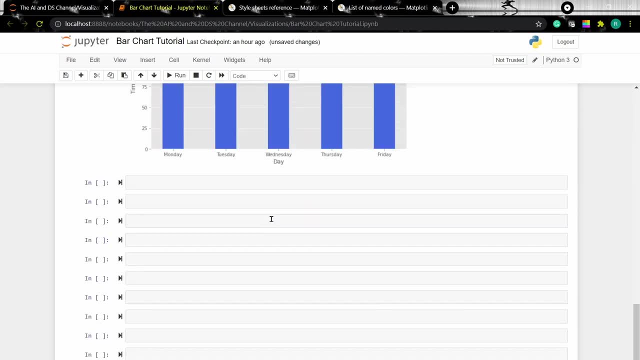 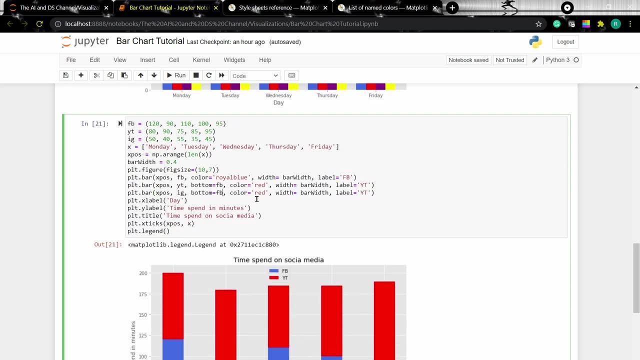 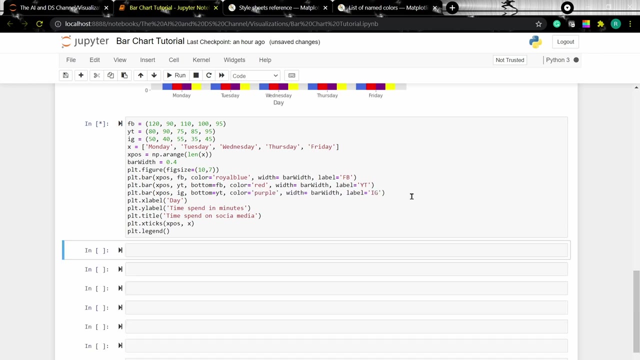 Now let's add a third bar to this. So I'm modifying the data over here. so the bottom of the third bar will be the top of the second bar. that is yt. change the color and if you run the cell, we have a stat bar chart. now let's look at plotting data from a csv file. 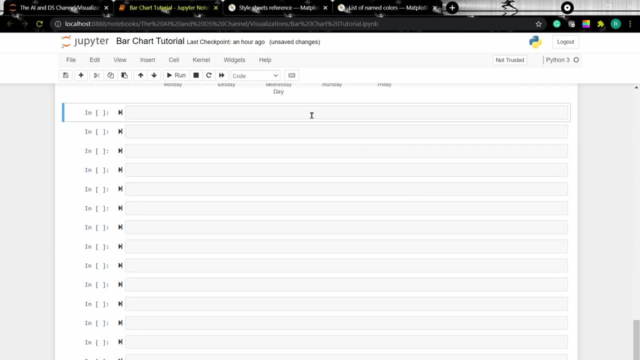 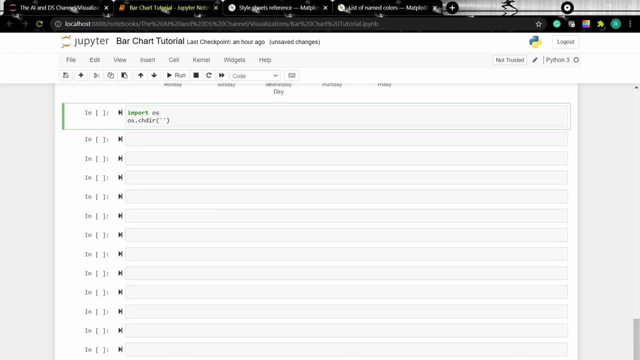 now, since we have already imported pandas, i'm just changing the part directory to know more about the pandas library. you can check out my previous tutorial on this topic. i'll add a link to it in the description below and the path where our csv file is stored. 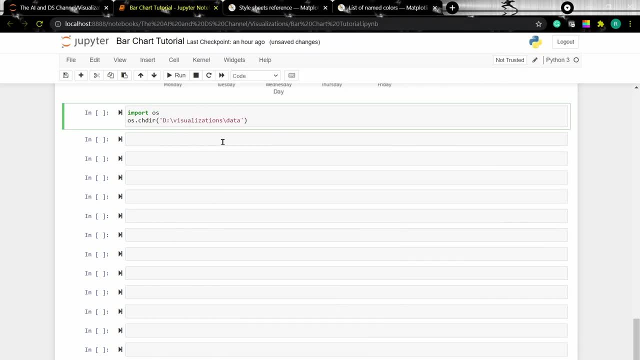 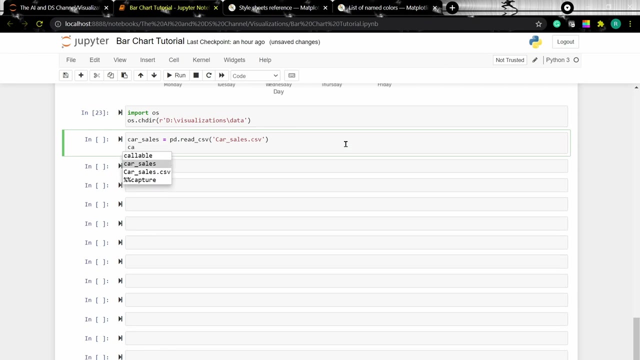 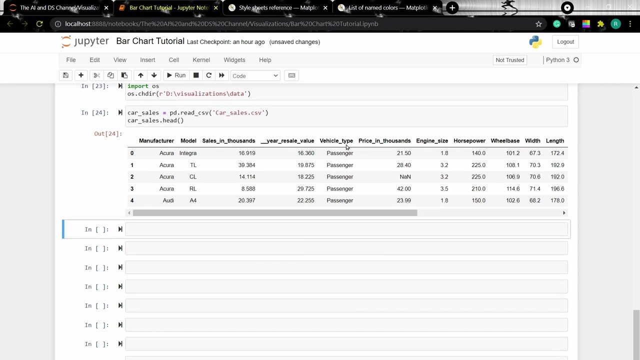 now let's read the data and create a data frame to see the data. we can use the head function now, from this data, we are going to plot a bar chart with the manufacturer and the sales. so to do this, let's create a variable to store the list return from the required columns. 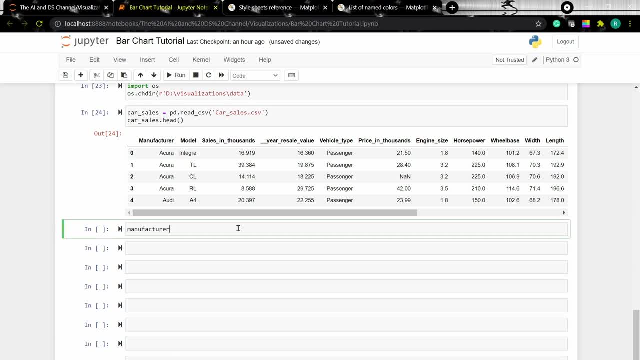 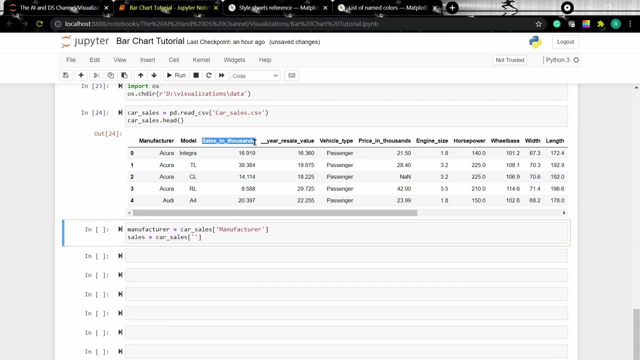 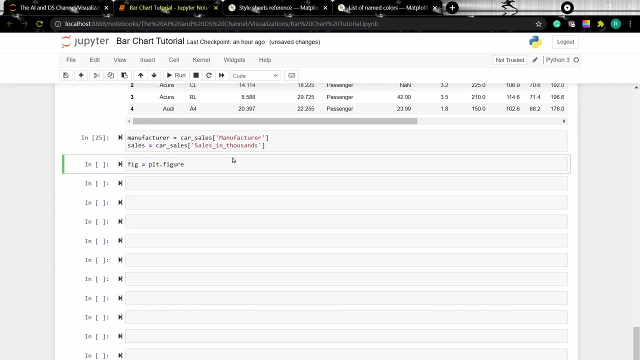 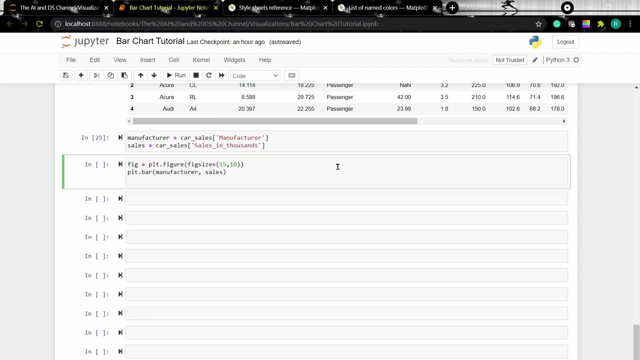 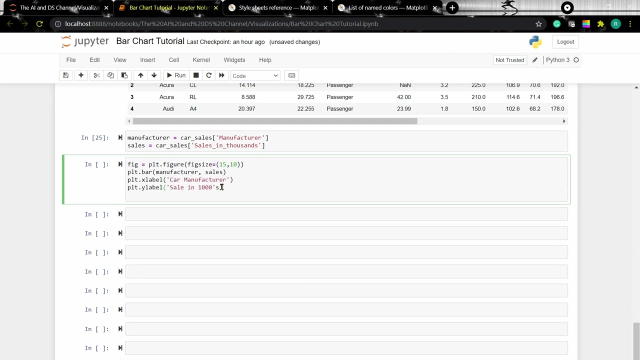 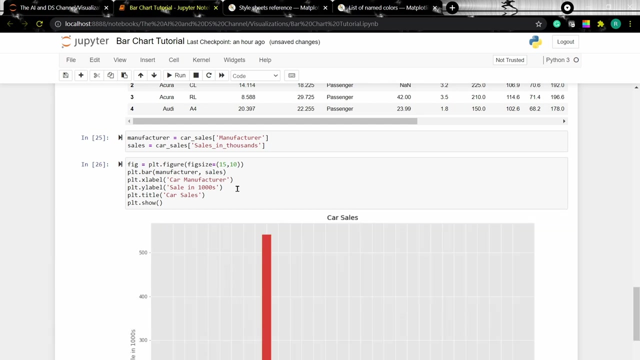 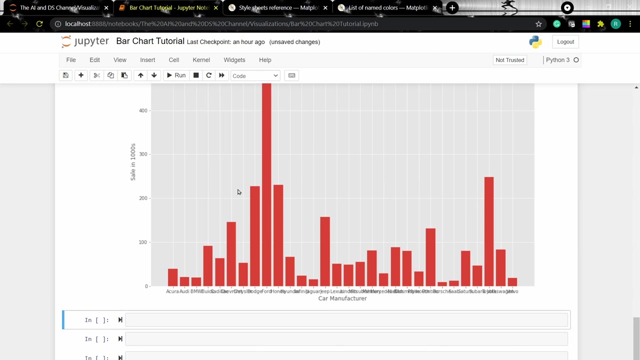 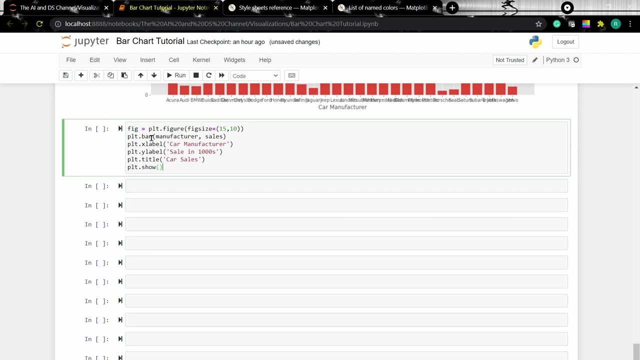 which in this case, is manufacturing sales. now let's plot the data. let's add the x label, y label and the title. now our data is plotted, but we cannot see the data labels properly. so let's make it into a horizontal bar chart. so, to make it into a horizontal bar chart, we can just replace the bar by. 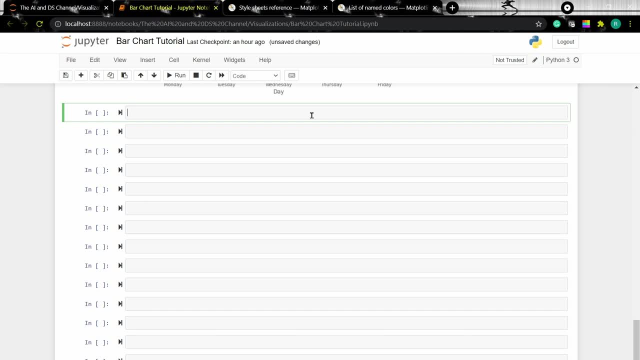 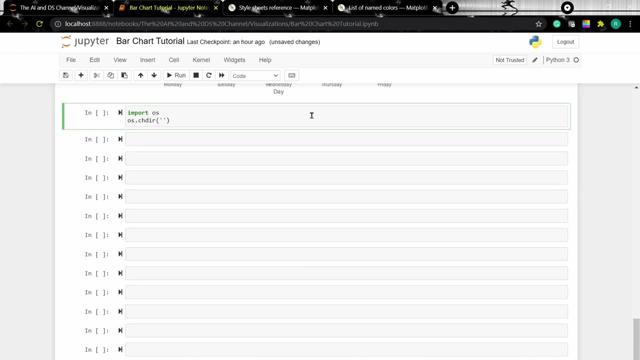 going to create a data frame. To know more about the pandas library, you can check out my previous tutorial on this topic. I will add a link to it in the description below And the path where a csv file is stored. Now let's read the data and create a data frame. 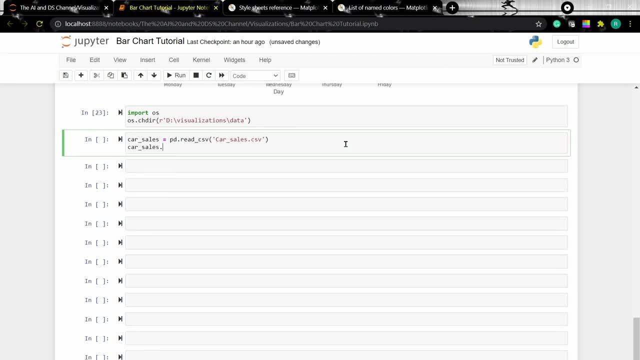 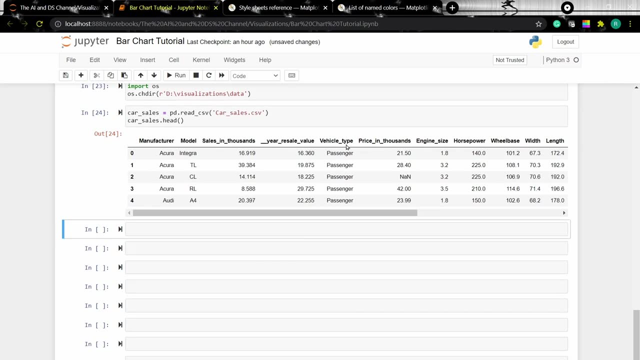 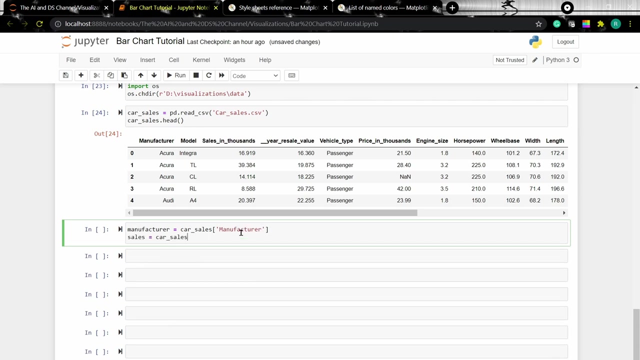 To see the data, we can use the head function. Now, from this data, we are going to plot a bar chart with the manufacturer and the sales. So to do this, let's create a variable to store the list returned from the required columns, which in this case is manufacturer and sales. Now let's plot the data. 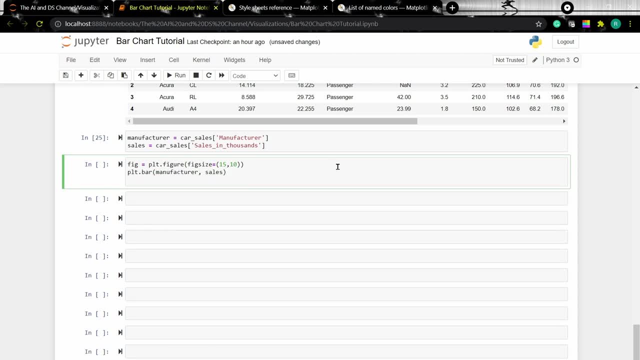 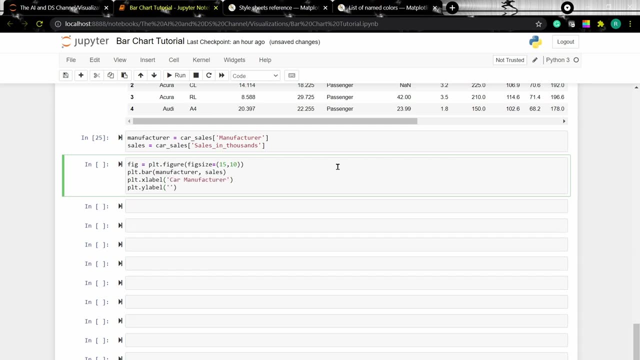 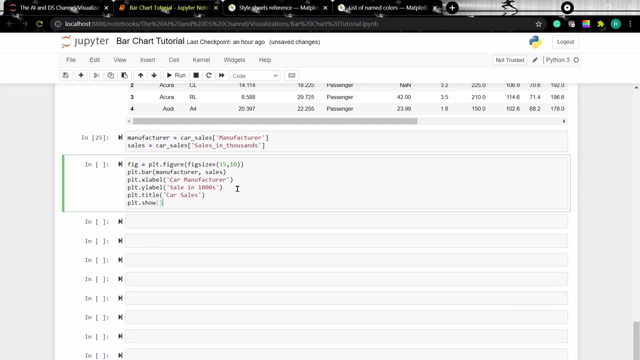 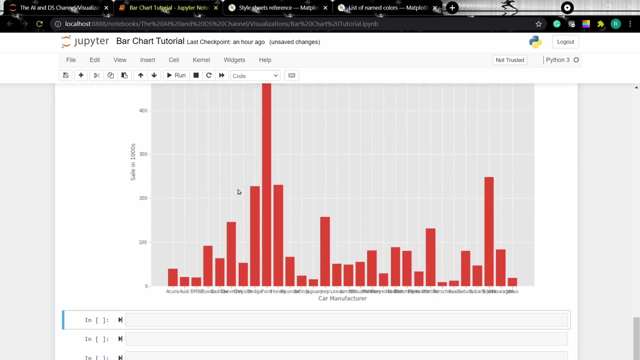 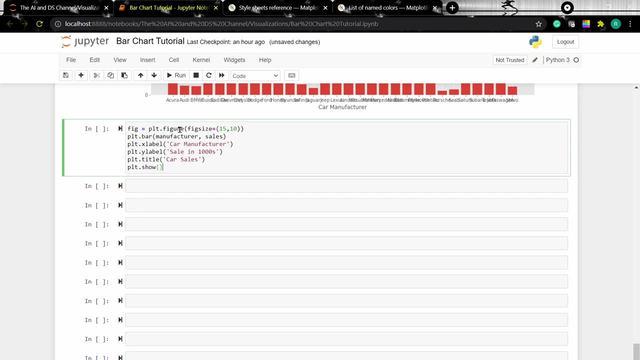 Let's add the x label, y label and the title. Now our data is plotted, but we cannot see the data labels properly, So let's make it into a horizontal bar chart. So to make it into a horizontal bar chart, we can just replace the bar by bar h and I. 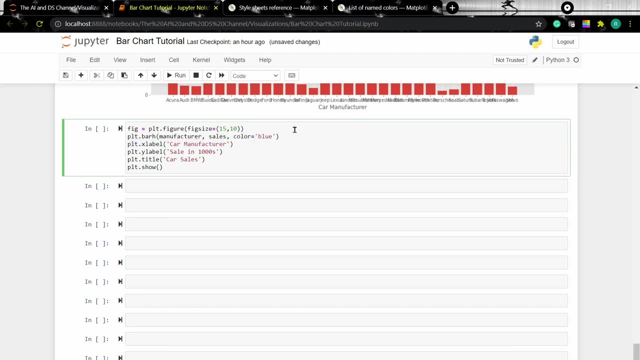 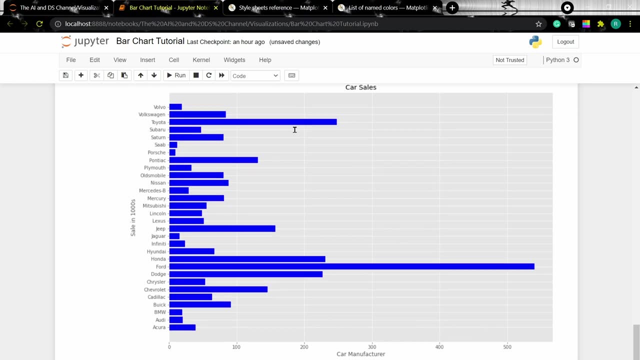 will also change the color. So now we have a horizontal bar chart and this is more readable. Now let's look at how to create a horizontal stat bar chart. For this, I am going to plot the fuel efficiency and fuel capacity of various car models from a particular car manufacturer. 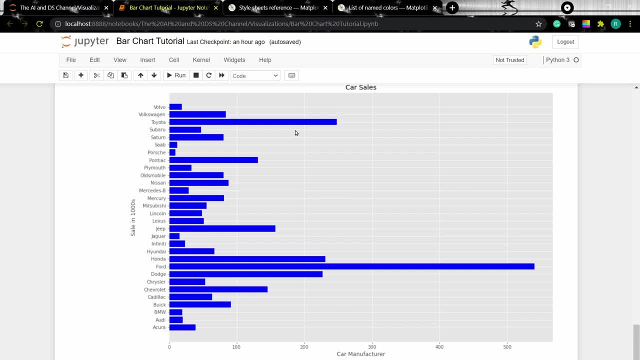 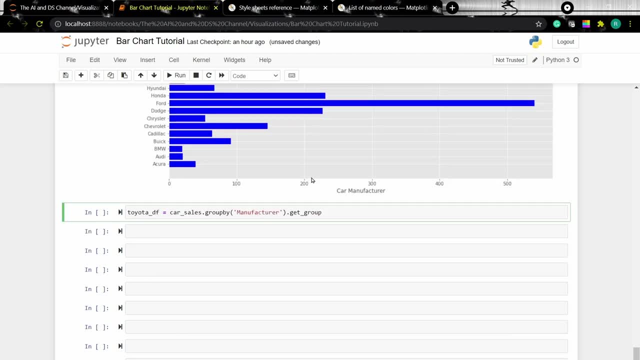 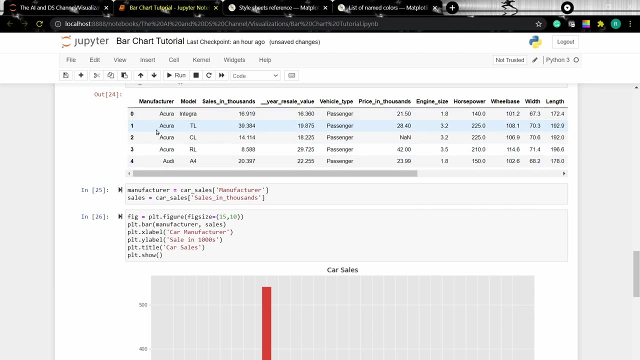 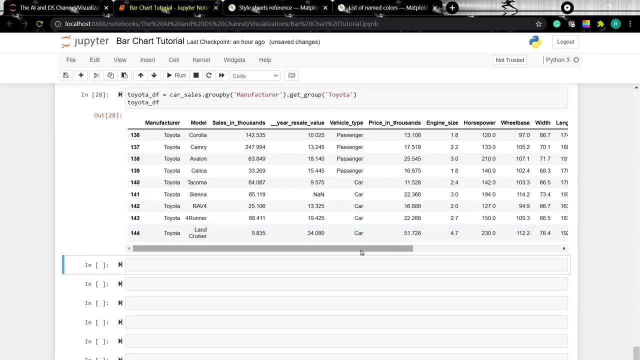 Say, for example, Toyota. So let's create a data frame to get the required data. So what this will do is it will group our data by the manufacturer column and then get the group which has labels Toyota in it To see the data frame we can type in: Toyota DF. 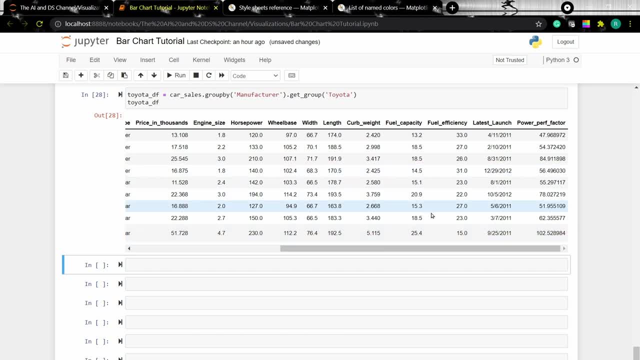 Now we need to plot the fuel efficiency and fuel capacity of the various Toyota cars. So to do that, we need to get the data frame. So I am going to plot the fuel efficiency and fuel capacity of the various Toyota cars. Now let's create a field graph for each car. 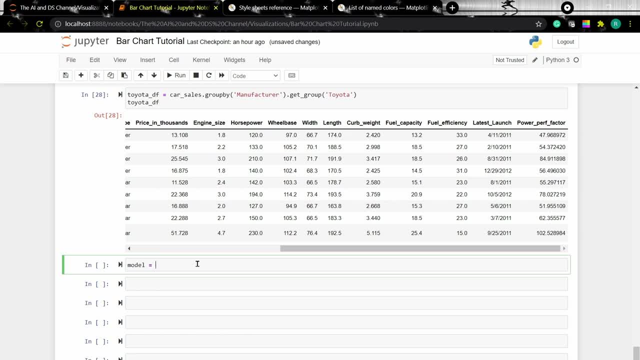 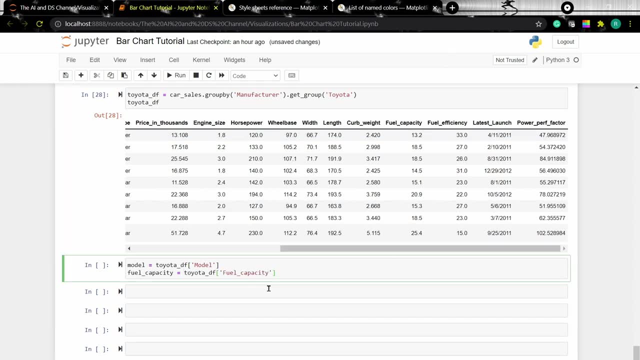 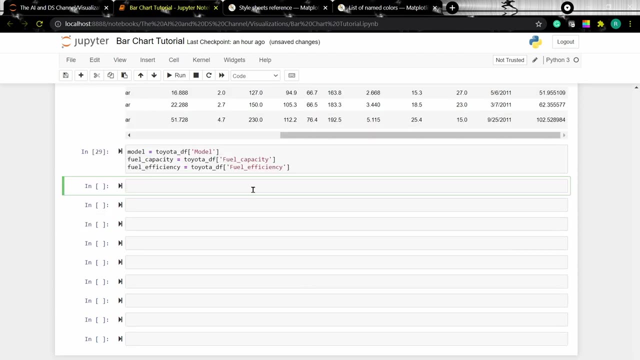 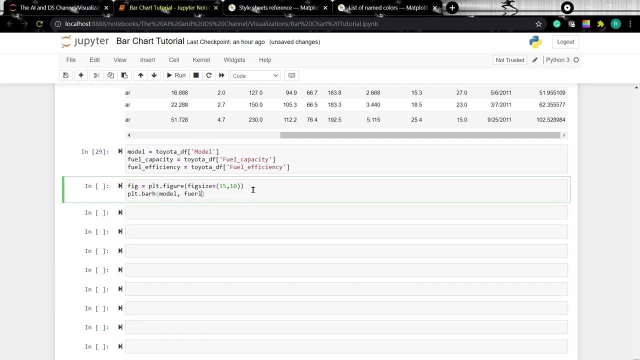 So from here, let's add the fuel efficiency and fuel capacity of the various Toyota cars. Now, to do that, we need to get the value. here required data. let's create variables for that, the model. now that we have a data, let's create a horizontal stack plot bar edge for horizontal bar chart for a. 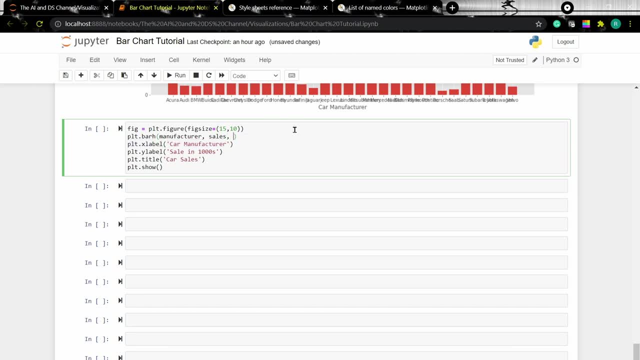 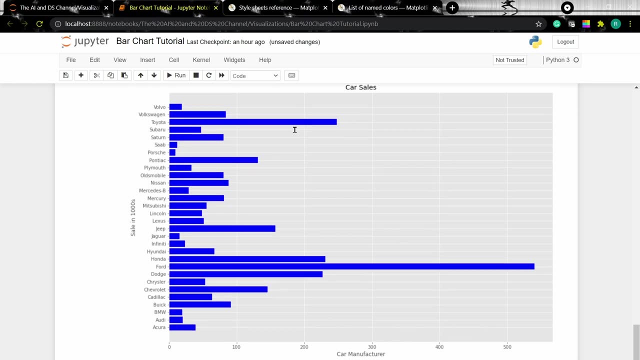 bar h and i'll also change the color. so now we have a horizontal bar chart and this is more readable. now let us look at how to create a horizontal stack bar chart. for this, i'm going to plot the fuel efficiency and fuel capacity of various car models from a particular car manufacturer. 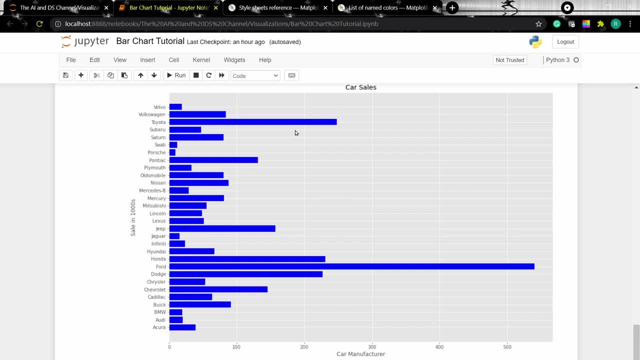 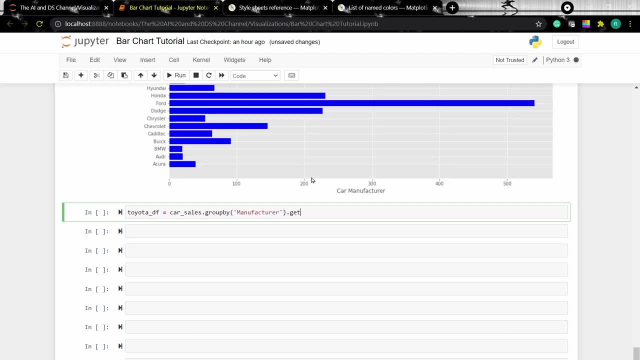 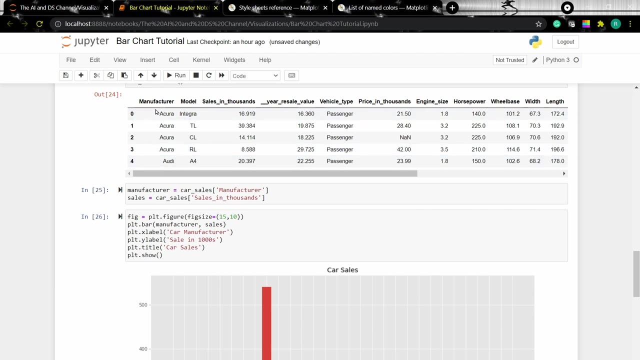 say, for example, toyota. so let's create a data frame to get the required data. so what this will do is it will group our data by the manufacturer column and then get the group which has labels toyota in it. to see the data frame we can type in: toyota tf. 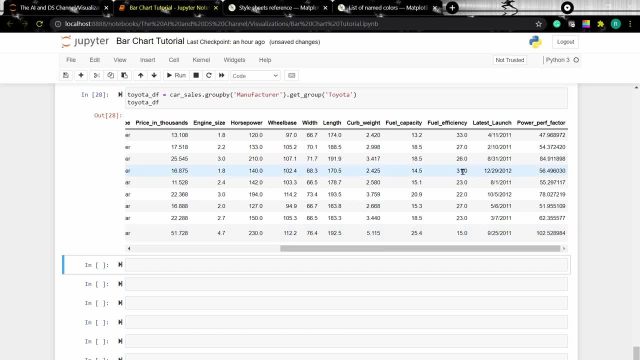 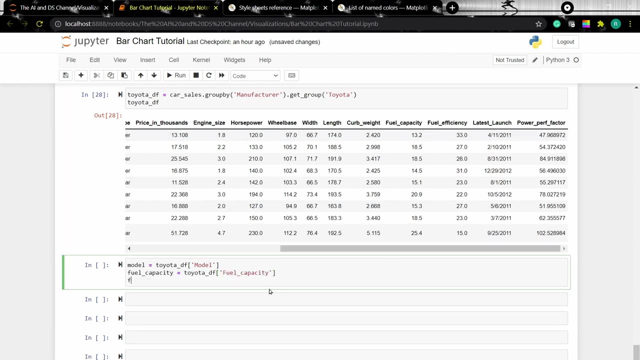 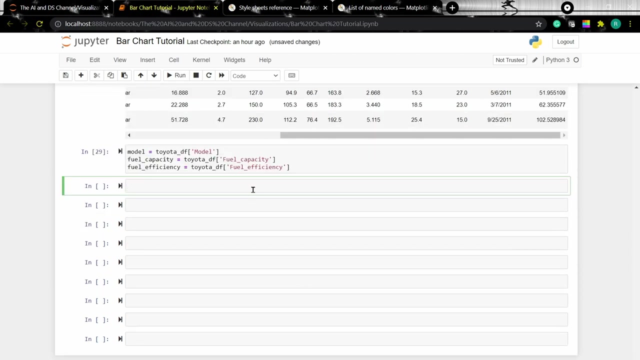 now we need to plot the fuel efficiency and fuel capacity of the various toyota cars. so to do that, we need to get the required data. let's create variables for that, the model. now that we have a data, let's create a horizontal stack plot. bar h for horizontal bar chart. 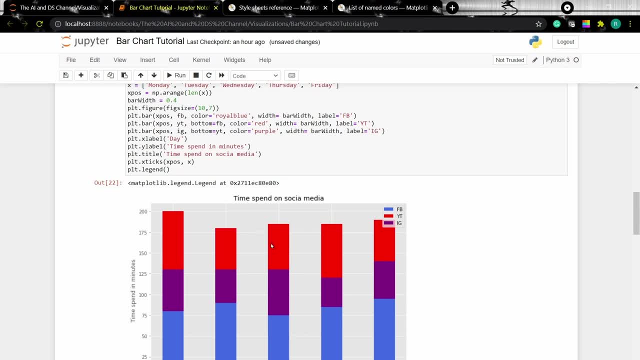 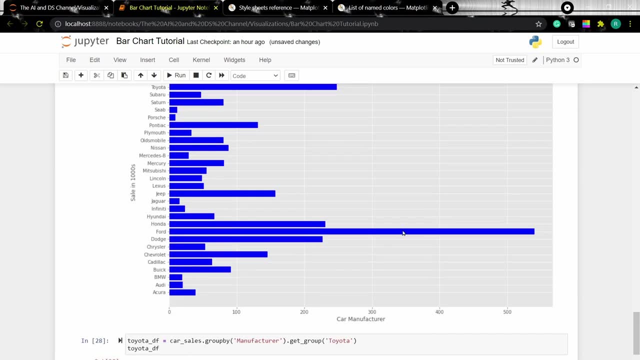 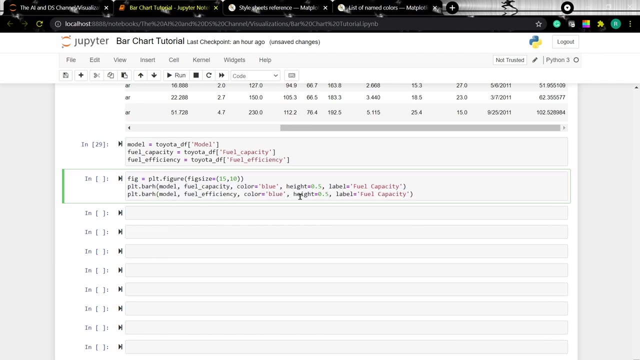 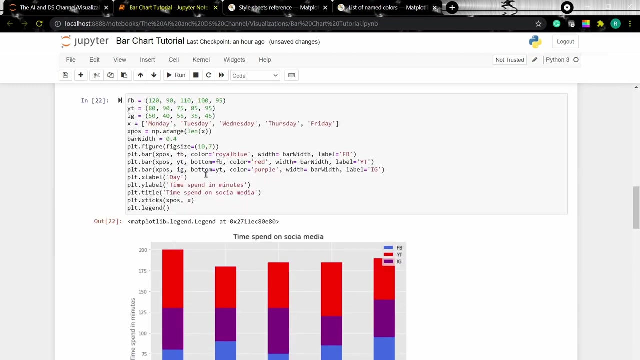 for our vertical bar charts, we needed to specify the width of the individual bars. for horizontal bar chart, we need to specify the height of the bar. this is the height of the bar- and similarly, for plotting a vertical stack bar chart, we need to specify the bottom position. 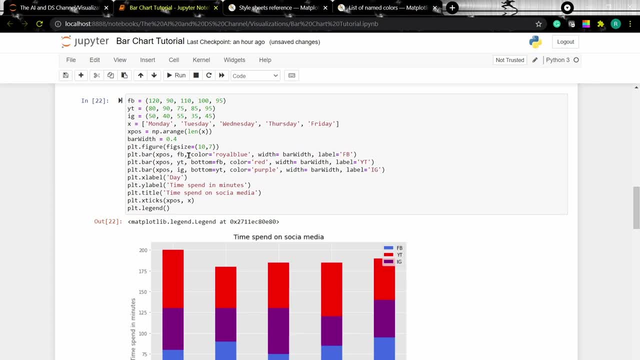 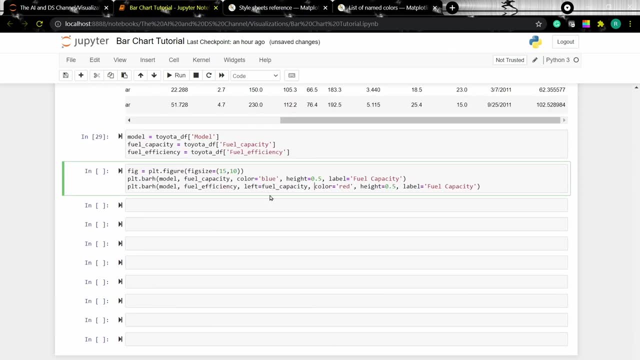 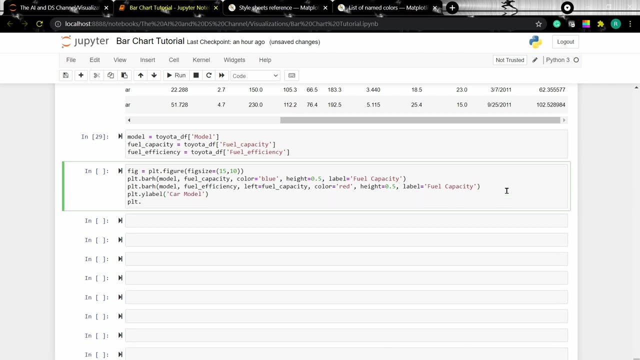 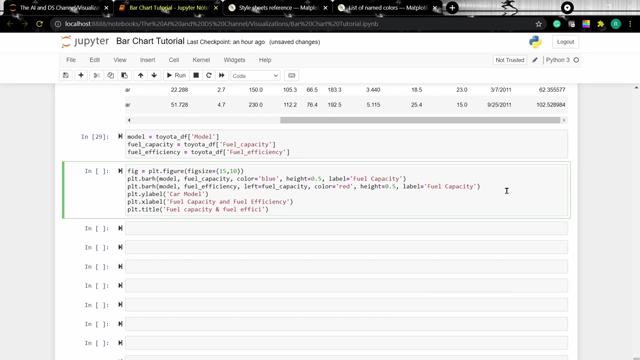 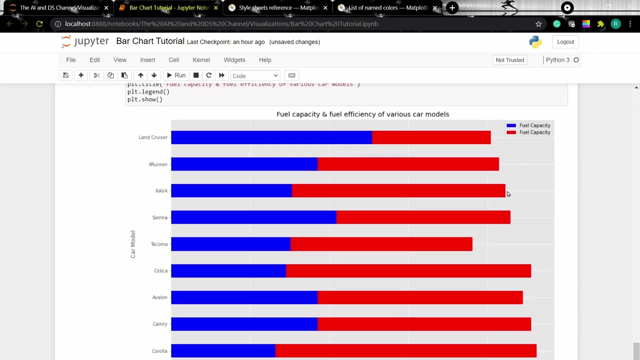 that is the bottom of the second data will be on the first data for a horizontal stack bar chart, we need to specify the left value, so what this will indicate is the left side of fuel efficiency will be fuel capacity and we have a stacked horizontal bar chart. that's all for this video. don't forget to like and share. 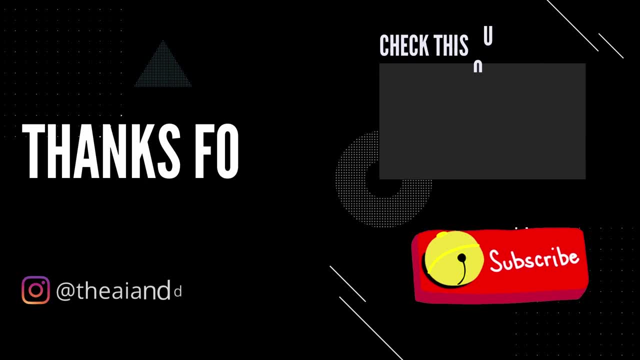 this video with your friends and family. so until we meet again in the next video. bye, bye video. if you found it useful, hope you got an idea about creating bar charts using matplotlib. let me know your thoughts in the comment section below. thank you for watching and see you in the next. video.